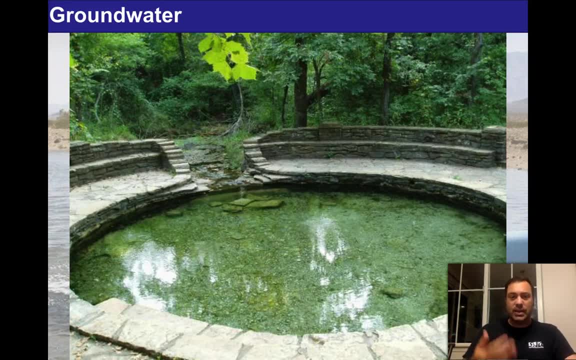 Why do these things happen? Why is this here? Why is it constantly feeding this water out? That's what this little lecture is going to be all about. You can see, this is a place that people built up, an area. I believe that people come here for some type of spiritual healing and they bathe in the pools. 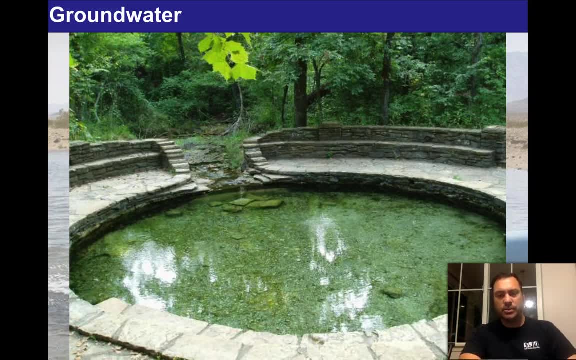 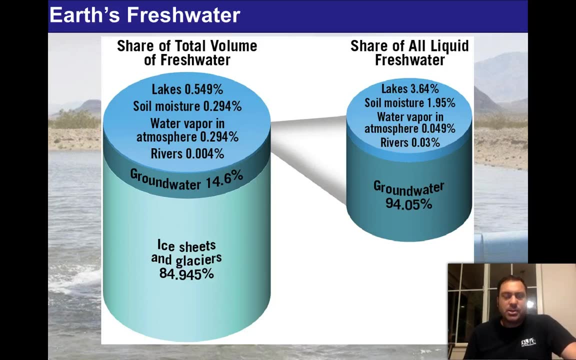 But anyways, you can see the benches here. These are for humans to use. So let's review where we were in terms of the amount of fresh water on the planet and how much of it might in fact be groundwater, why we're talking about it so much. 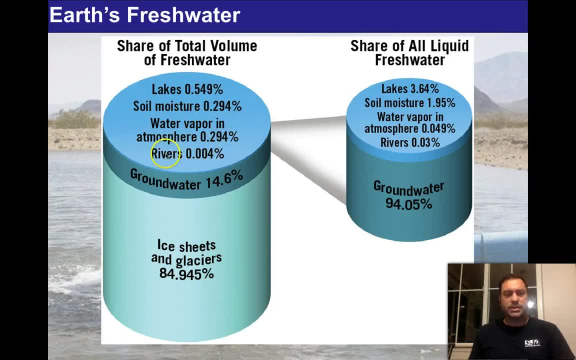 Well, the total volume of fresh water, and of course, fresh water being a very small percentage of the water on Earth. if you don't remember that conversation, go back and view the previous lecture. But we have lakes at half a percent of the total fresh water. soil moisture, you know, maybe a quarter of a percent, a little more. 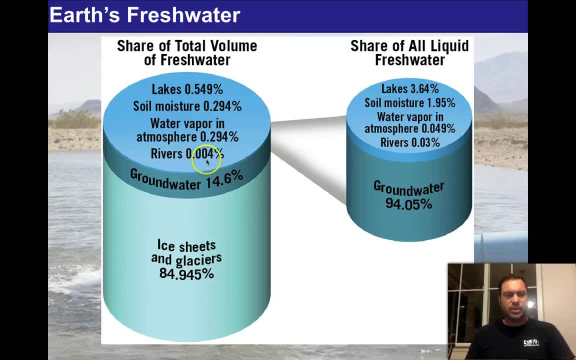 Water vapor is about a quarter, And rivers is an extremely small. four- that's tenths, hundredths, thousandths- that's four thousandths- of the total fresh water in the world is in rivers at any given time. Look at this. Groundwater, though, is 14.6 percent. That's a sizable amount. 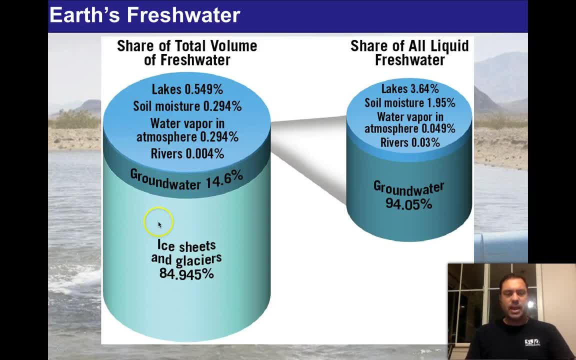 So we've talked about this stuff here, but we haven't talked about this yet, And one of the upcoming lectures- I believe actually the next one- will be ice sheets and glaciers. We'll be talking about this one here, So let's go ahead. 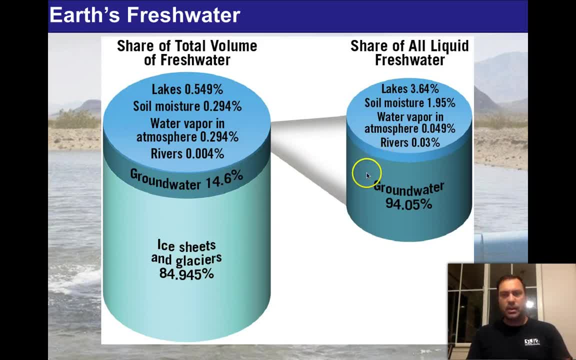 Jump right in and talk about groundwater. Now, groundwater itself: in terms of all liquid fresh water, okay, which is to say, taking out the ice sheets and glaciers, which are solid fresh water, groundwater is 94.5 percent, by far the largest amount. 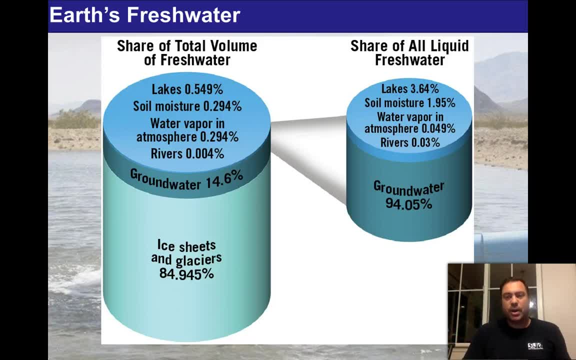 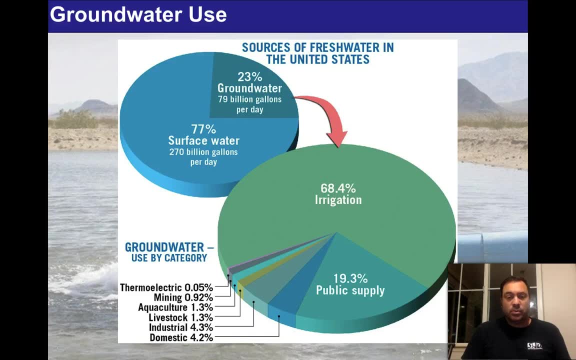 And that's why we care so much about it. Of course, to exploit groundwater, we're going to need some technology. We're going to talk about the science behind this in a moment. So, in general, we need to ask ourselves: what do we do? 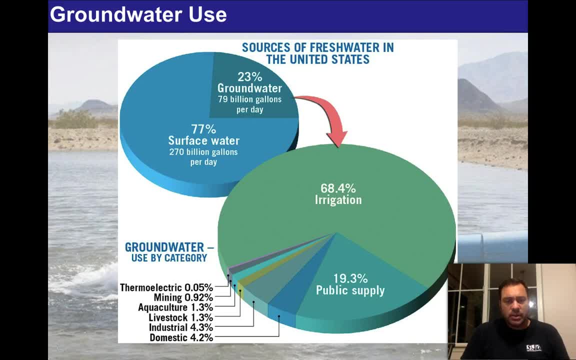 What do we do with the groundwater? What is the use for it? Well, to understand that question, we need to look at a couple of pie charts. I've got here, So, sources of fresh water. in the United States, most of the fresh water that we use is actually the surface water. 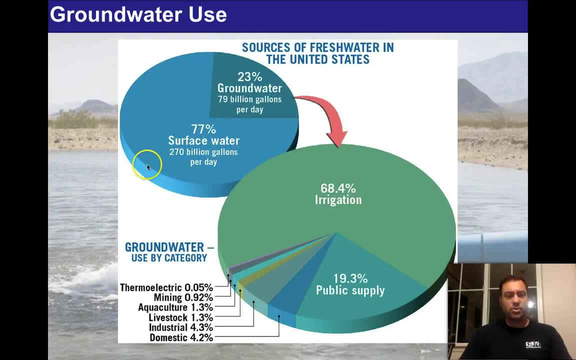 But remember, surface water is really a very small percentage. The majority, 95 percent of usable water is actually groundwater And that's about 23 percent of the consumption that we do on a daily basis: 79 billion gallons as of right now. 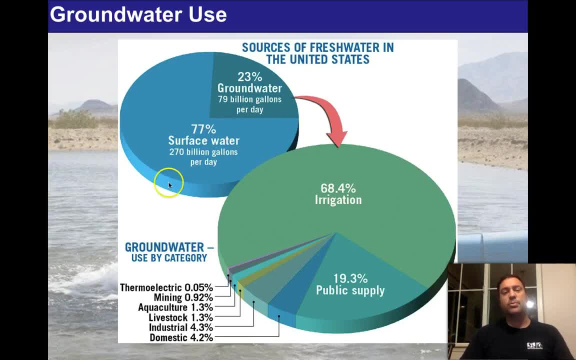 And how much of this is usable. And what it should say is: how do we use this very large sum, 270 billion plus 79 billion gallons per day? Well, 68.4 percent of it is used for irrigation. Far and away most of it is used by farmers to grow food or to grow crops. 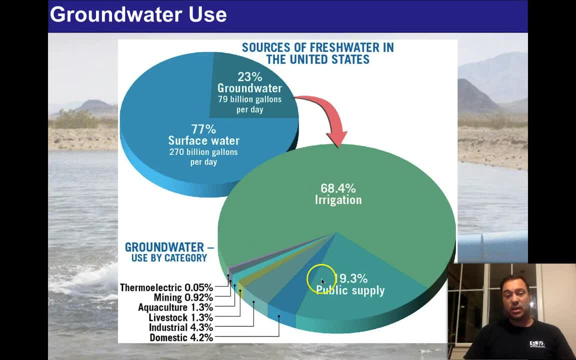 But we also use it for other things. Public supply, which means watering your lawns, washing your dishes, just drinking water, is 19.3 percent. That's the public supply. I should say Domestic supply 4.2.. 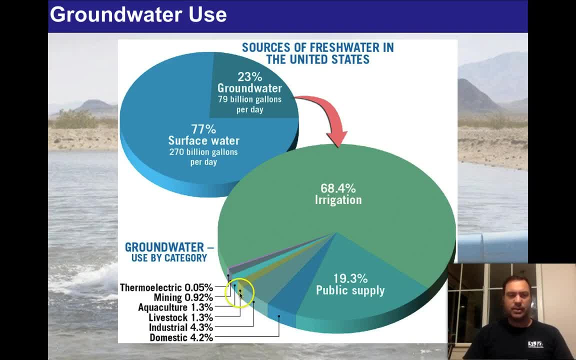 Industrial, 4.3. Livestock. you know you've got to feed the cows and the aquaculture and mining and thermoelectric. You get the idea. There's a lot of different places that we use the water. 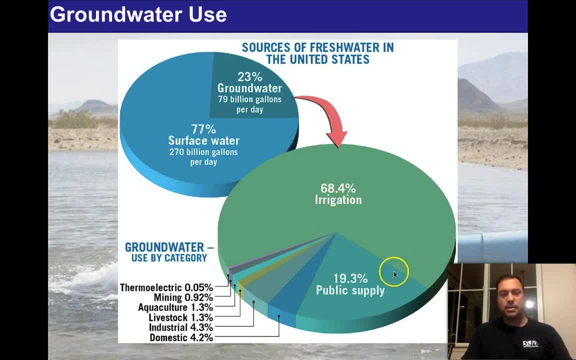 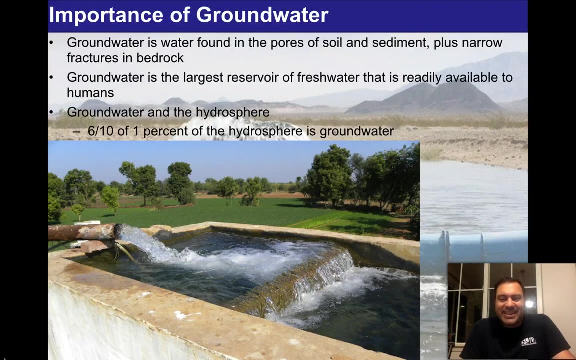 But far and away these are the three major areas: the irrigation, the public supply and the domestic supply, So used by municipalities such as cities, used by farmers and used by homes. So where is groundwater then? You know, obviously it's in the ground. 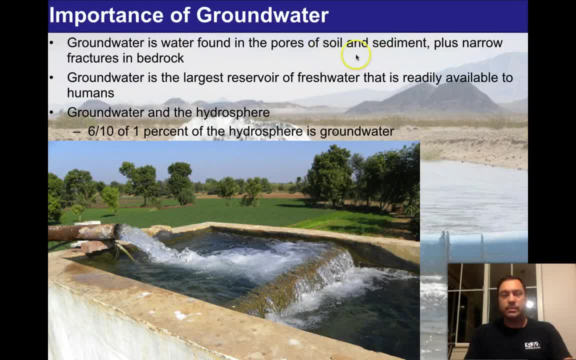 But groundwater is basically found in the pores of sediment and soil, plus narrow fractures in bedrock. You'll have to review some of the previous lectures if you don't know what I'm talking about: the pores of soil and sediment. Review the lecture on sediments and how rocks form and they'll talk about how soil and water interact- or, I'm sorry, sediment and water interact to percolate fluids through and to cement things up. 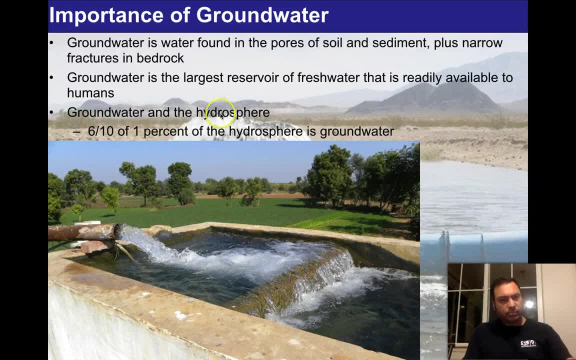 But it's the open space, That's what a pore is, And groundwater is the largest reservoir of freshwater that's readily available to humans right- 95% almost. But of the total hydrosphere, six-tenths of 1% of the hydrosphere is groundwater. 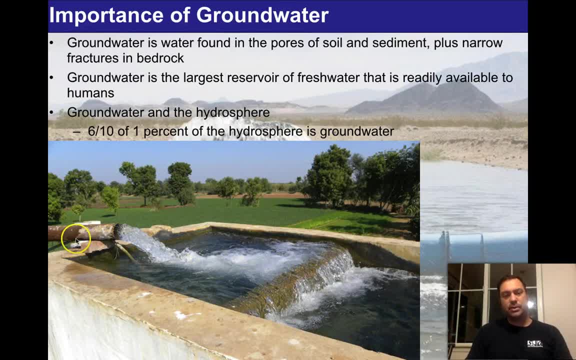 So we have to take out, you know, of course, the ocean or whatever, And here we see a groundwater, pumping water in. This is for an agricultural area. here This is an agricultural field. here This water is pumped out of the ground and literally put right into the field. 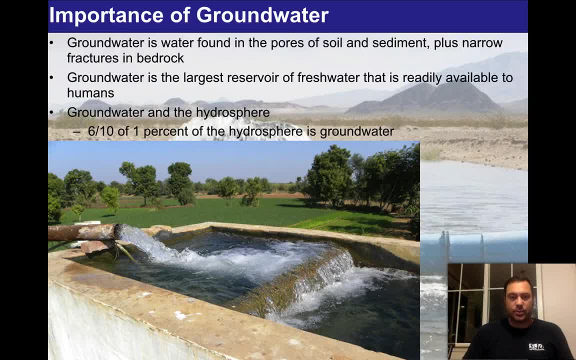 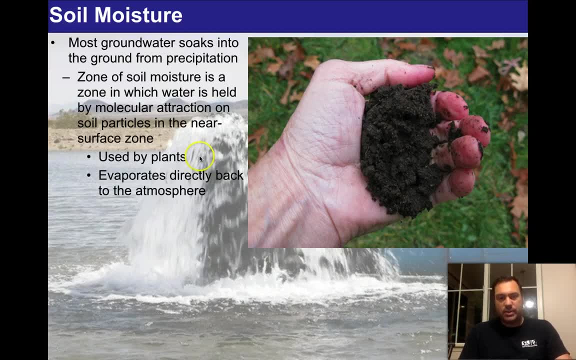 There's no treatment or anything Like that. It's usually used right out of the well, So most groundwater finds its way. There's a couple of ways that it finds its way in, But most groundwater soaks into the ground from precipitation. 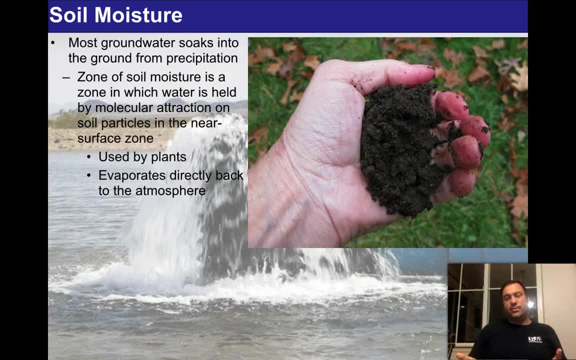 In other words, the source of the water is usually rainfall or snow melt or something like this, And it basically comes straight down and it soaks into the soil and eventually makes its way down, So there's usually a zone of soil moisture, that is. 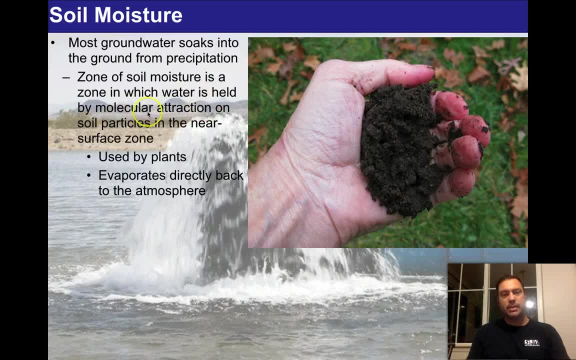 Held basically in the soil particles, by molecular, by molecular attraction. So the water comes in and basically it wets the grains of the sediment within the soil And this is really kind of neat because it makes it usable by plants. Otherwise it'd go all the way straight down. 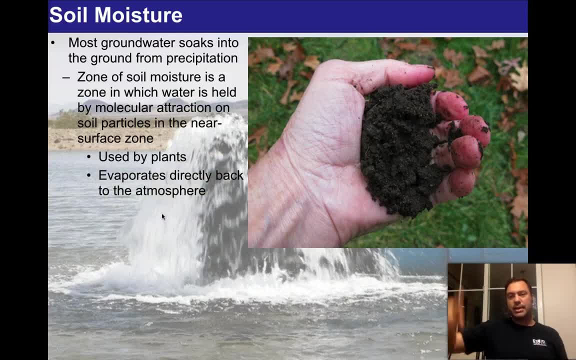 It also evaporates directly back into the atmosphere, So it's watch a cycle with the atmosphere itself. So when the sun is out, it'll evaporate. when this, when the clouds return, it'll actually get wet again and cycle back around. 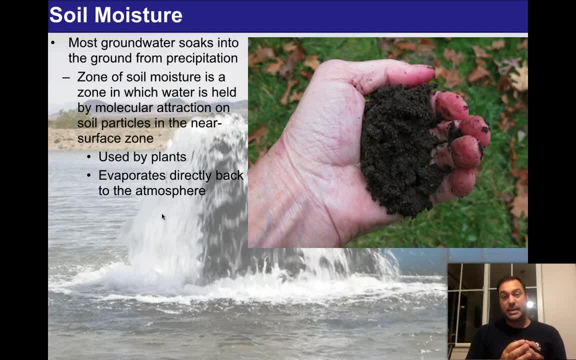 Of course the plants Do the same thing. It uses the water and uses it in its metabolism and returns the water back to the air. So it cycles around in this way, But of course not all of it makes its way out. 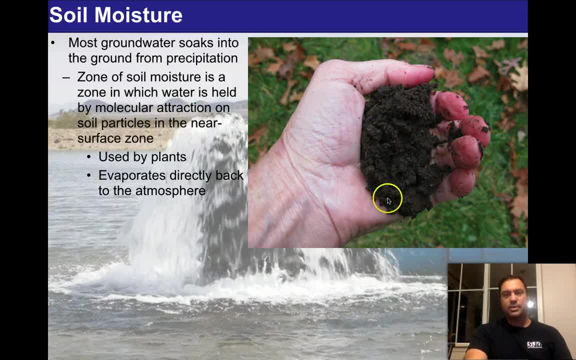 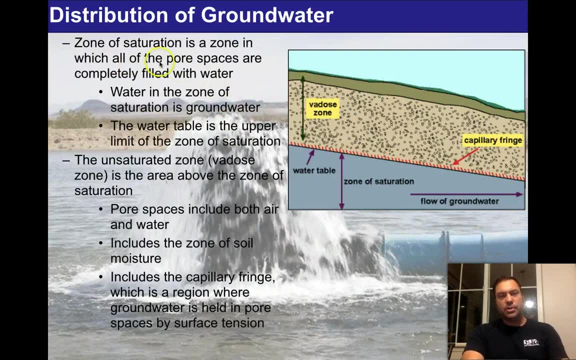 So this is kind of a typical after rain: soil, The nose. It's pretty wet here. So the distribution of groundwater. There's a couple of little buzzwords we're going to bring in here, but there's something called the zone of saturation. 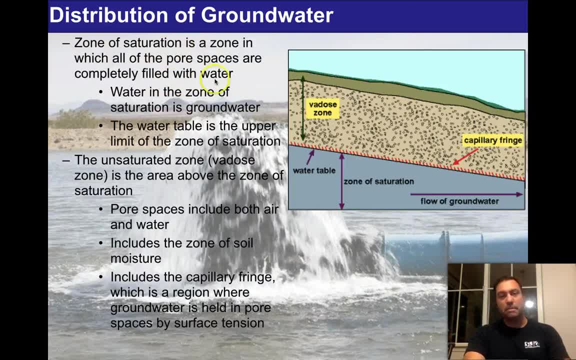 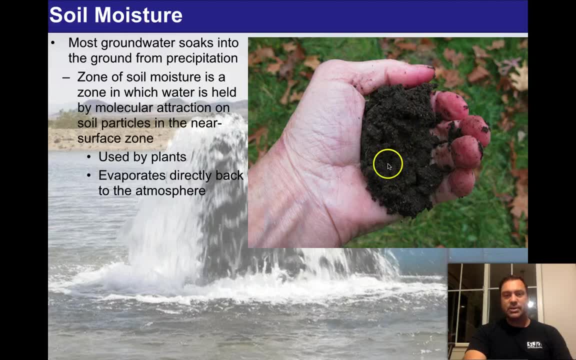 So the zone of saturation is a zone in which all of the pores Spaces are completely filled with water. So back here- this isn't the soil up here is in a zone that is not necessarily saturated, It's still. it's basically the water sticking to the mud, but there's still air in there. 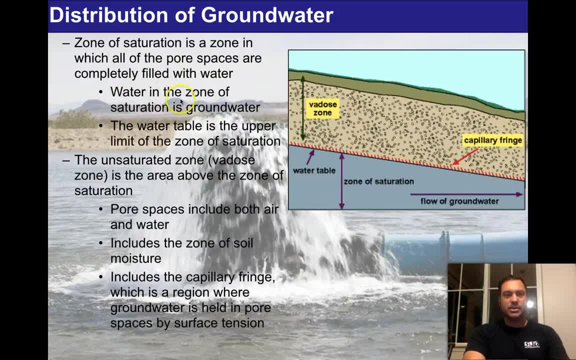 There's still open space. This is what they're saying here- is is that there's a zone of saturation where the water has completely replaced all the air. There's no open space. OK, so water in the zone of saturation is groundwater by definition. 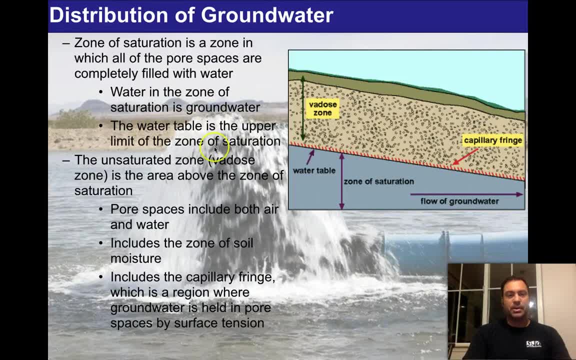 That's what We're calling groundwater, and the water table is the upper limit of the zone of saturation. So you can imagine if you have a bunch of sand in a bucket and you start pouring water into that bucket, the water is going to make the sand on top wet. 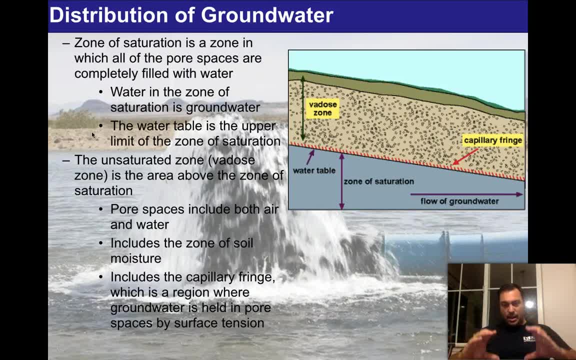 But it's all going to pile up at the bottom of the bucket right up to a certain level, and that water that's piling at the bottom is basically the saturation zone. That's the groundwater. Everything above it still might be wet, but that's unsaturated. 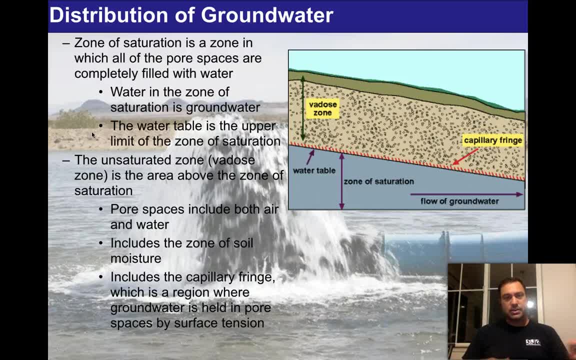 There's still water, but there's also air. next, OK, this is talking about the zone of saturation. So water tables do the same thing, So here would be a zone of saturation. This is a land surface. up here. The unsaturated zone is the area above the zone of saturation. 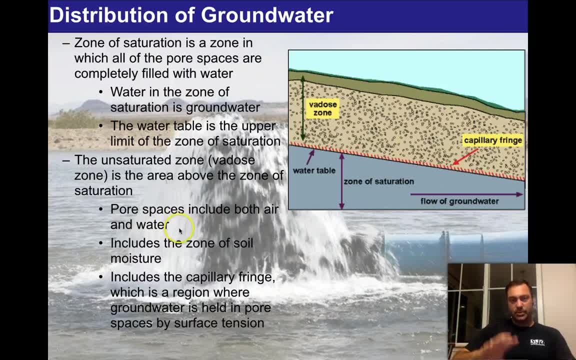 So pore spaces include both air and water. in our former examples that are the upper section, And so that would be something. By the way, the unsaturated zone is also called the Betos zone, And so here's the Betos zone, right here up on top. 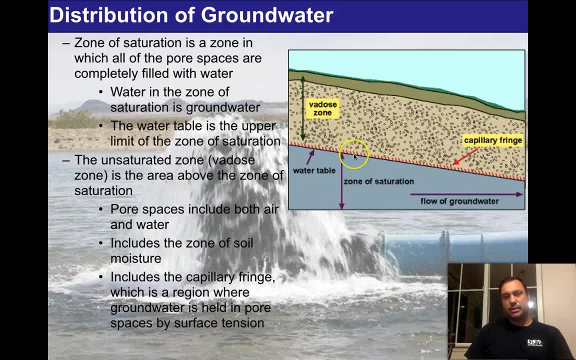 And so the water basically rains into the top, soaks in and goes right down To below the water table. the water table is basically the uppermost point at which there's no air. right up in here There's still some air in the in the rocks includes the zone of soil moisture. 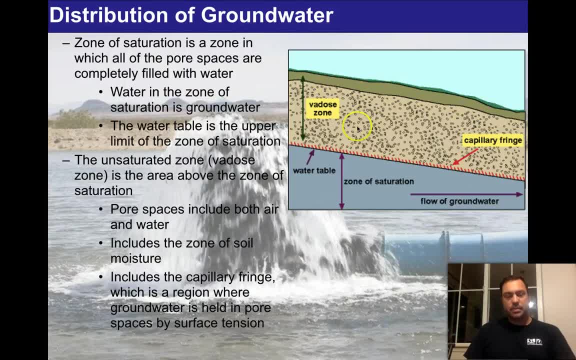 So there's a soil moisture zone right up here, This green area right here which is not marked. it includes the capillary fringe, which is a region where groundwater is held in pore spaces by surface tension. So there's a zone here. 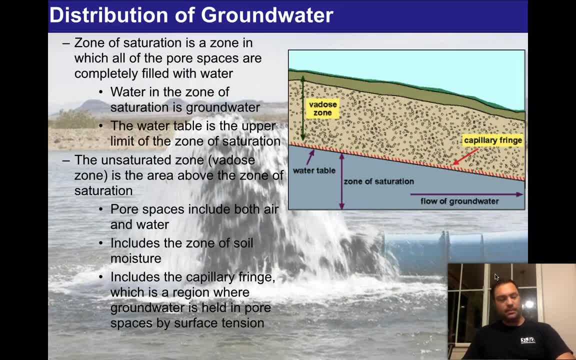 We got the water table and Some of you have seen this- or actually I'm pretty sure almost everybody has seen this- that if you take a piece of paper, you stick it in water, the water starts to crawl up the paper and soak the entire thing. 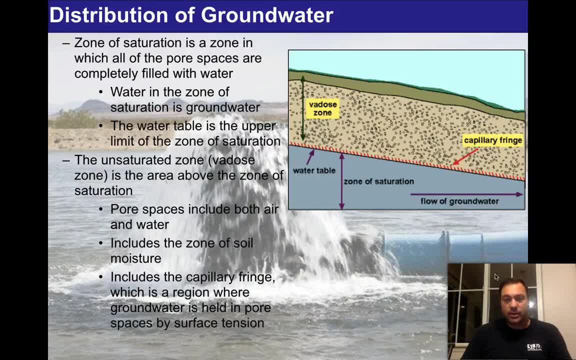 And basically that is a surface tension feature. I'm not going to get into the details of the physics of it, but starts to climb up, And so you get paper and water in that situation. Well, it does the same thing in soils and in rocks. 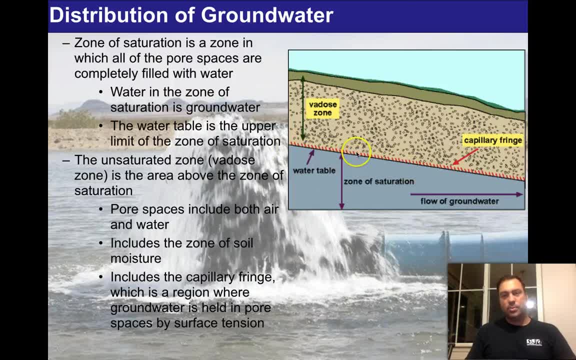 It turns out that if you have a nice water table, the water will start to Climb up from the water table up into the unsaturated zone or the beta stone, and that's called the capillary fringe, because something called capillary action- now in this case the flow of groundwater is from left to right- will describe the reason why. 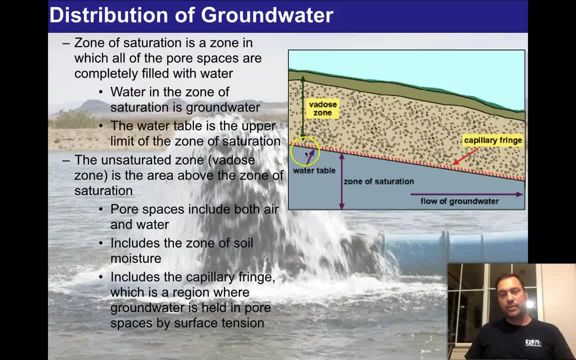 But you could tell that it's going to be predicted that we have a gravitationally high area and a gravitationally low area, and usually go from areas that are high to low naturally. So the water is basically moving to the right, All right. 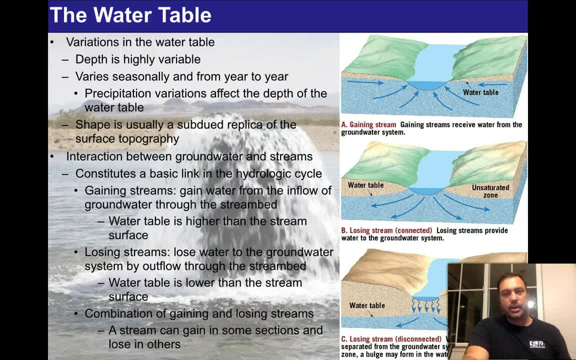 So this is kind of a neat little little diagram right here, the position of the water table relative to different features on Earth's surface. Well, first off, depth is highly variable. You can go to different places on and look at different rocks under the water table and you'll find that sometimes those rocks are affected deeply by the water table and sometimes they're not touched at all. 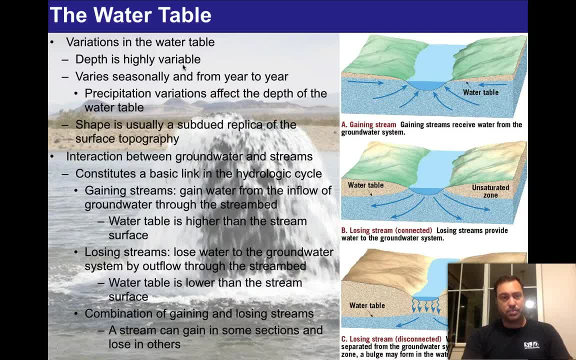 There's geologic reasons for this. We're going to basically try to break this down in a very simple Five way. First off, the depth to the water table. very seasonally and from year to year, Right So, in the summer months, where it's drier in some areas, the water table might be very low. in the winter months, where it rains a lot, could be very high. 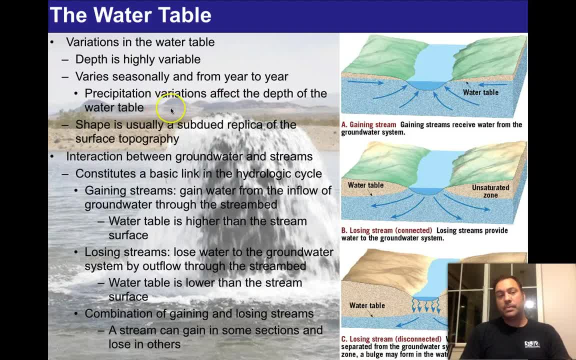 So precipitation variations affect the depth of the water table and the shape tends to to follow the subdued or to produce a subdued replica of the surface topography. In other words, the water table tends to go up where there's a hill and go down where there's a valley. 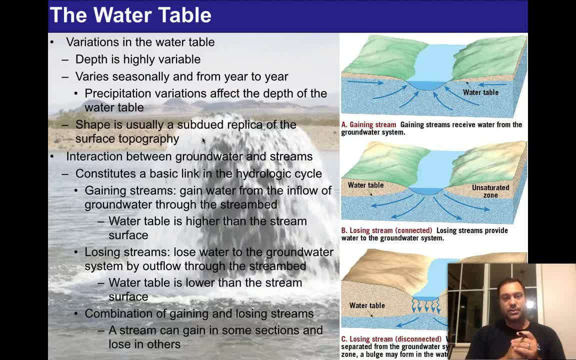 It basically kind of rides along with the surface features of the earth. Now there's a couple of really cool things that are going on here. First off, the interaction between groundwater and streams is extremely important, because when we were talking about surface water before, we were ignoring the groundwater issue. that's going on there. 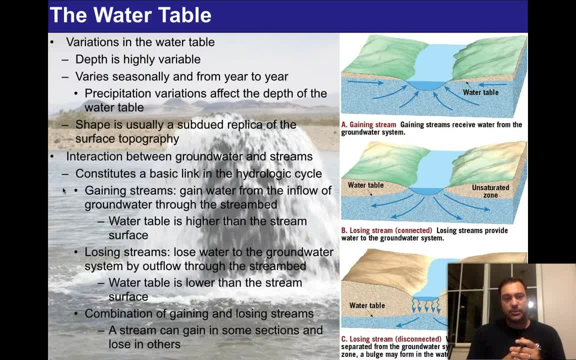 We were just talking about how water moves across the surface and how the sediment moves, But we didn't really talk about what happens when the water, or what happens to the water in a stream itself when it runs across, Say, a Sand or a bunch of rock fractures. 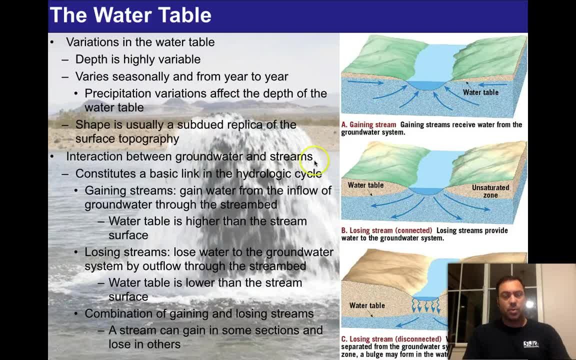 OK, Well, there's a major link that occurs between groundwaters and streams. So this is, and in fact it's, a basic link in the hydrologic cycle. So gaining streams are are a type of system where the water would. they gain water from the inflow of groundwater through the stream bed. 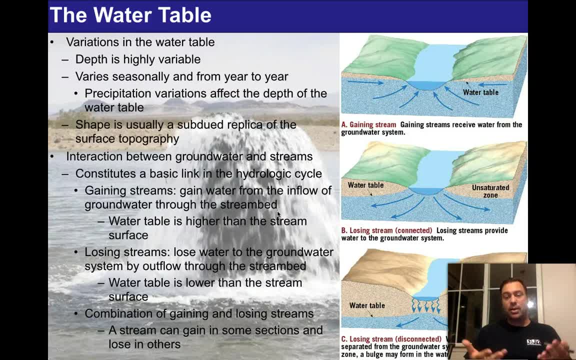 So water comes constantly. There's so much water in the groundwater aquifer that it dumps into the stream and it's transported out of the aquifer. In this case, Here's the water table: water table, The stream is cutting into the aquifer and are into the saturation zone. 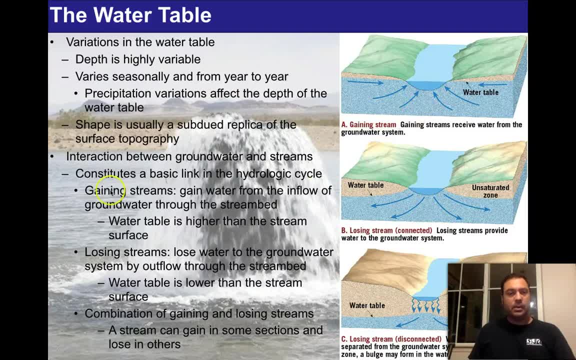 I'm sorry- and transporting it away. So, water, the water table is higher than the stream surface. when this happens, Right, This is what we see here. So, literally, the stream surface is forming the top of the water table, Losing streams. however, a situation where the where the water table is higher in the stream than it is in the rocks around it. 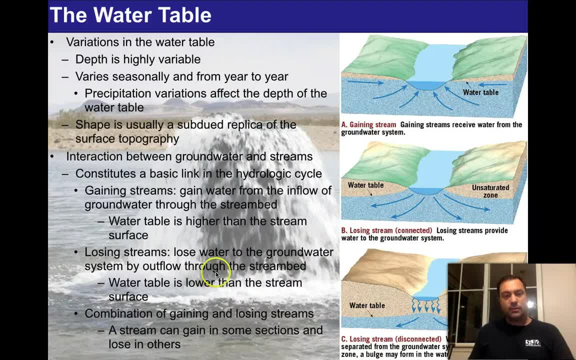 So these tend to lose water. Of course that's going to cause the water to flow through the stream system. It has to flow through the swimming system to the water system, to the river, to the groundwater system, by outfloat and stream, that, in other words, soaking in. 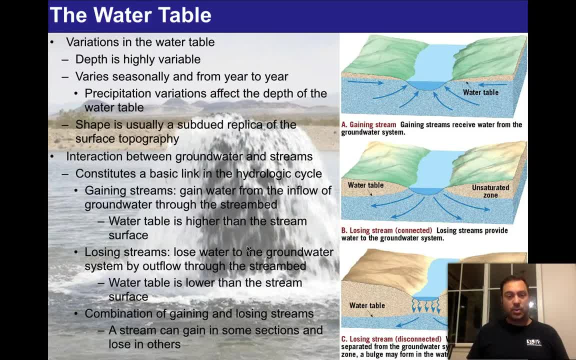 So the river is flowing in here And in this case, as it's flowing through it, soaking into the, Into the groundwater system, And so the river is actually shrinking away. In certain environments it may completely disappear. So in this case, the water table is lower than the stream surface. 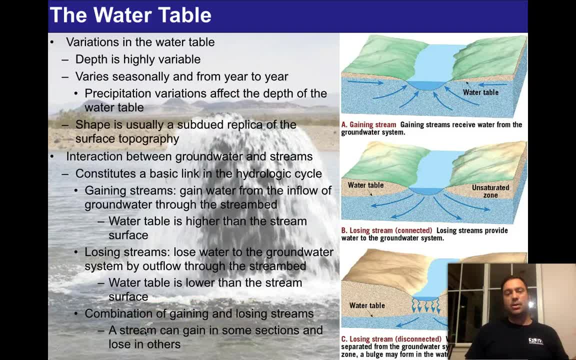 OK, so here's the water table. Nice and low Stream surfaces sitting up high, Of course, are not all one thing. Not all rivers are all gaining streams and all of them are losing streams, But I would say that the majority of the ones I have experience with personally- 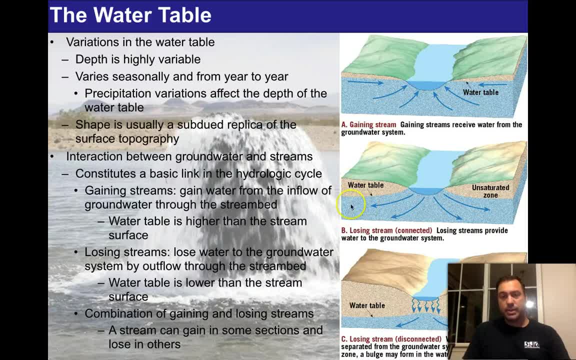 are gaining streams, But if you go out into certain desert environments, you see losing streams all over the place. Okay, so it really depends on a lot of different features, But it is important to know what it is you're dealing with. This is kind of a neat little thing. This. 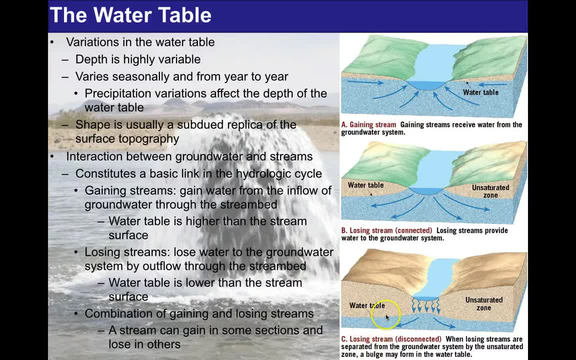 is a what they call a disconnected losing stream. So this is where the water table is so low relative to the stream that that very situation happens: That the unsaturated zone is actually connected underneath the stream And so it's constantly dropping water into the groundwater. 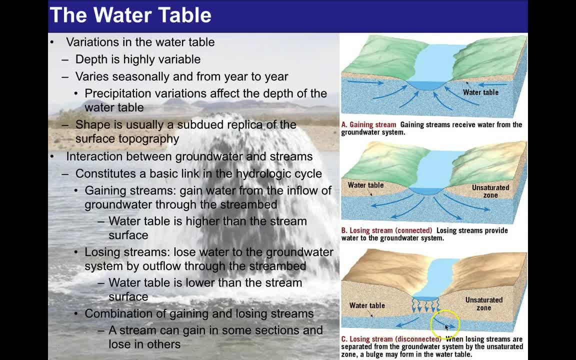 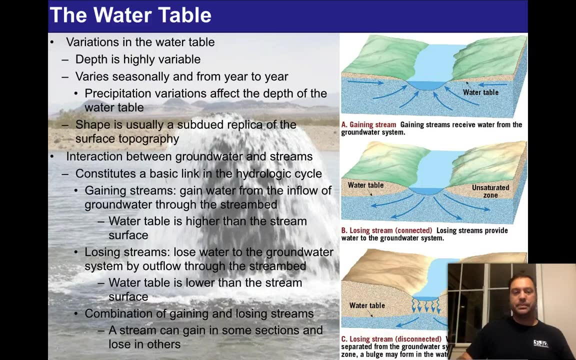 aquifer. Okay, so this creates a bulge on the aquifer without at the same time connecting the surface- I'm sorry, the water table- with the stream itself. So this is kind of a neat thing. This is what you see typically in certain desert environments. 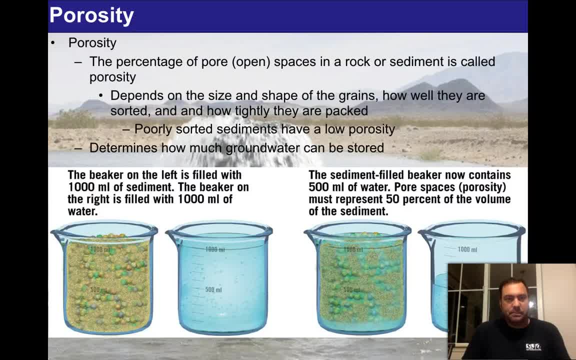 Alright, so let's talk about some concepts. Porosity: We've talked about porosity before, but this is kind of a neat little thing that we need to talk about in more detail. So porosity is the percentage of open spaces or poor spaces, air open space right in a rock or sediment. 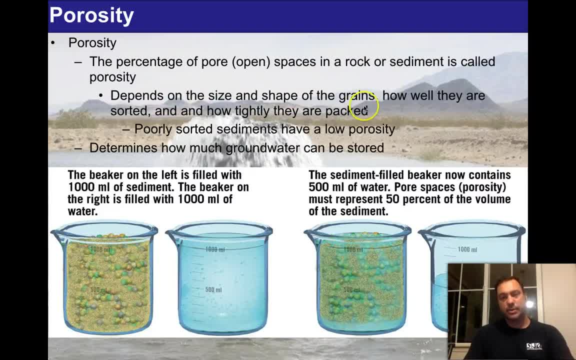 And that's called the porosity. It depends on the size and shape of the grains, right? Some things like clays tend to tend to fill in holes really well, whereas sand grains tend to have large holes, And so it's kind of a neat little thing. So porosity is the percentage of 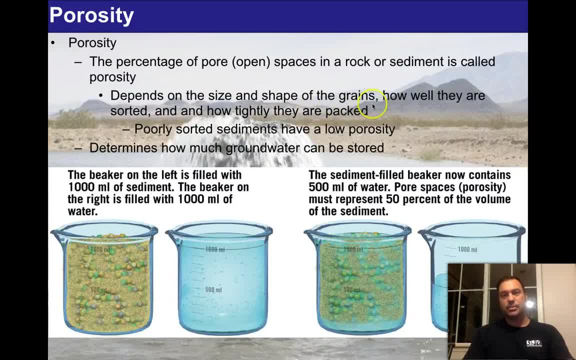 open spaces or poor spaces, air open space, right, And that's called the porosity And it around them. So it depends on the size and shape of the grains and how well they are sorted and how tightly they are packed right. You know, you can take a. 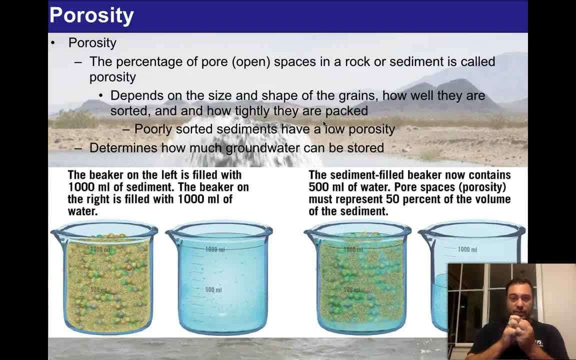 bunch of sand grains and have loose versus sand grains that are really tightly shoved together and that has an effect on the porosity. So poorly sorted sediments have a low porosity. it turns out right. So if you have a lot of large boulders and you have little bits of sand, the little bits of sand can fill in. 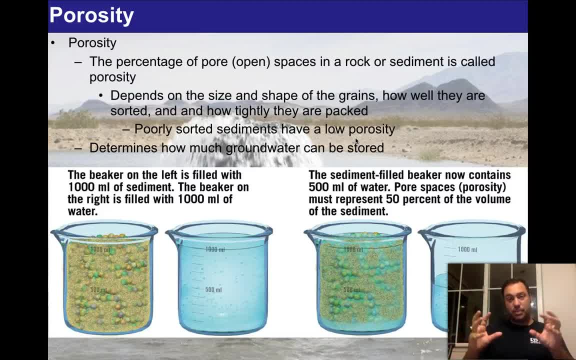 the holes left around the big boulders. But if you have nothing but nice big boulders, the water can get through very easily And of course the porosity determines how much groundwater can be stored right. That becomes the reservoir itself. So let's look at this example. We have a beaker on the left that is filled. 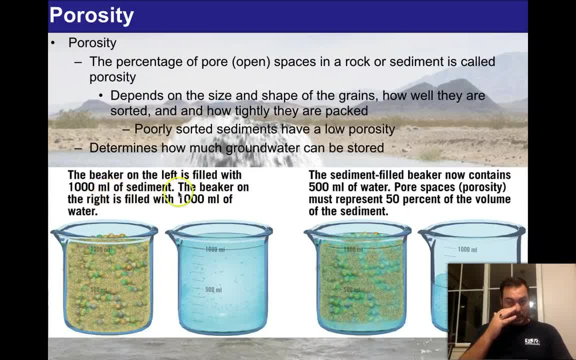 with a thousand milliliters of sediment. That's a standard liter. The beaker on the right is filled with 1,000 milliliters of water. right, They're equal amounts. okay, Here we see the sediment filled beaker now. 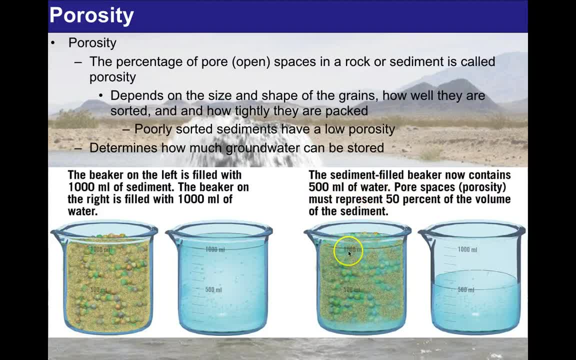 contains 500 milliliters of water. So they've taken 500 milliliters of water, they've dumped it in, right? What does that tell us? The fact that we're able to fill this up and it's dry? we're able to add 50, or, I'm sorry, 500. 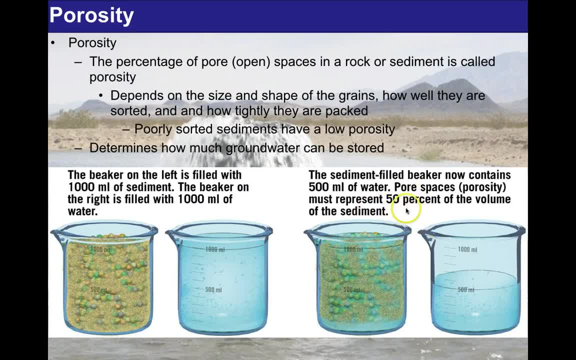 milliliters of water. Well, it means that the pore spaces must represent 50% or half of the volume of the sediment, because I'm able to take half of this and dump it in there and it fills in all the spaces. Kind of a cool little simple. 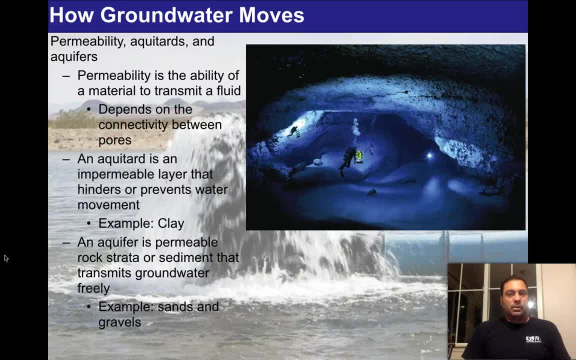 test that we can do So. how does groundwater move, then? right, We know that there's now there's open spaces, that there's water that can fill into the cracks or into the pores. What happens once it gets down there? Well, there's several things that we 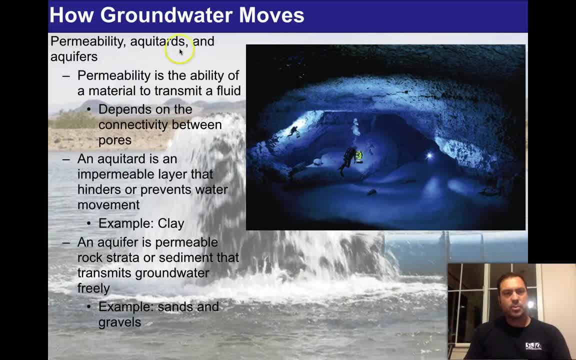 need to be aware of right Permeability, something called aqua tarps- we're going to talk about those here in a minute- and aqua furs. So permeability is the ability of a material to transmit a fluid, in other words, to shoot a fluid. 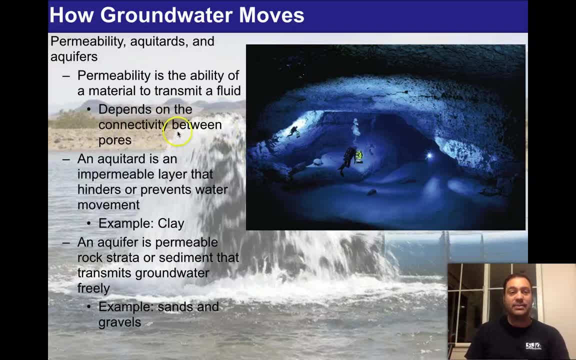 through the rock And it depends upon the connectivity between pores. So sometimes you have pore spaces that are really very closed up. So if you have a pore space that can hold a lot of water, but the water can't flow from pore to pore very 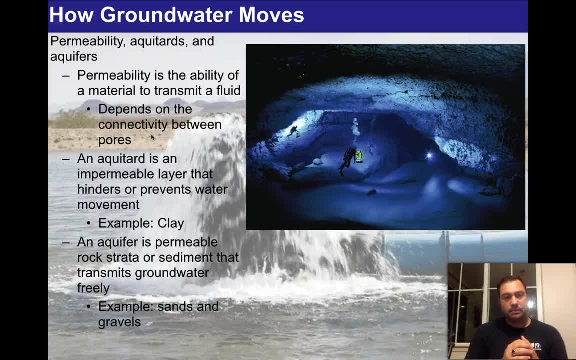 easily or at all in some cases. So that depends on a lot of things. Sometimes there's very good connectivity right. Water just goes through it very fast. As a matter of fact, here is a giant underground aquifer and here's a 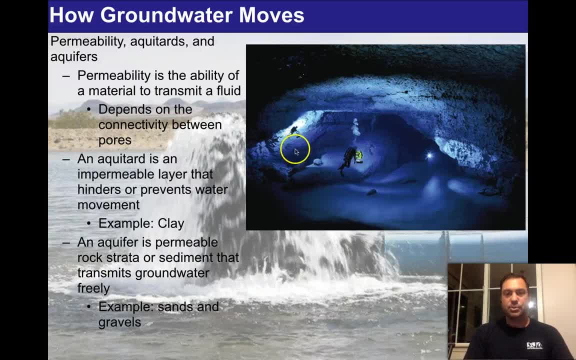 matter of fact, here's a couple of divers that are swimming in the aquifer. I believe this is a photo taken in Florida. This is one giant open pore Right. It's huge. It's the size of an undersea cavern. So, anyways, you get the. 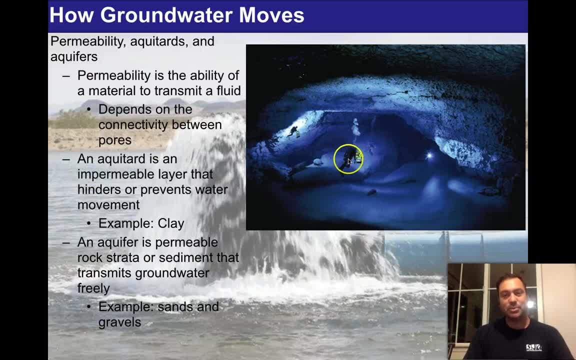 idea Highly connected in this situation, right, So so much so they could swim through it. An aqua tarp is an impermeable layer that hinders or prevents water movement, And clays are a typical example. right, They're really. 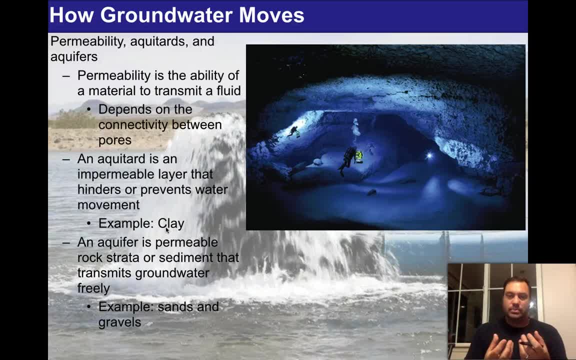 really small. They're usually poorly sorted. They're everything that water hates to transport through right. So clay is a really good aqua tarp So it restricts water flow. I'm sorry. an aquifer is permeable rock strata or sediment that. 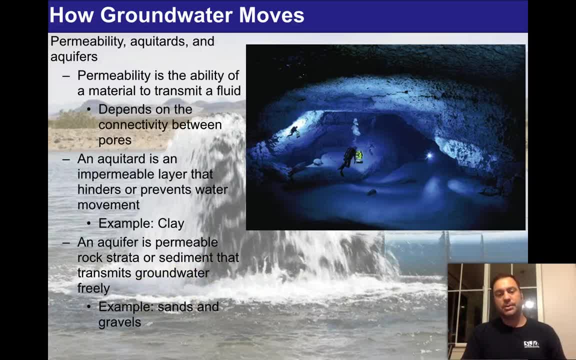 transmits water freely. The typical examples that we see in natural systems are sands and gravels. All right, So old stream beds that have been covered up over time become very, very good at transmitting groundwater- at very high velocities in some cases. And, of course, this environment here, which is called a 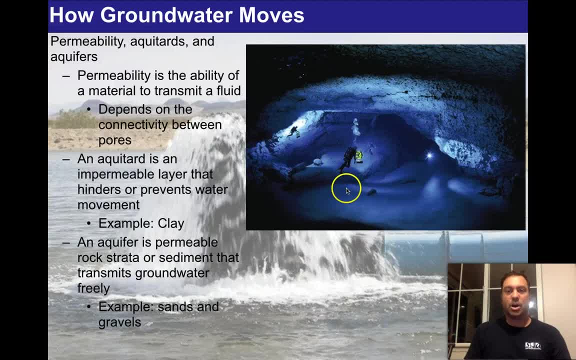 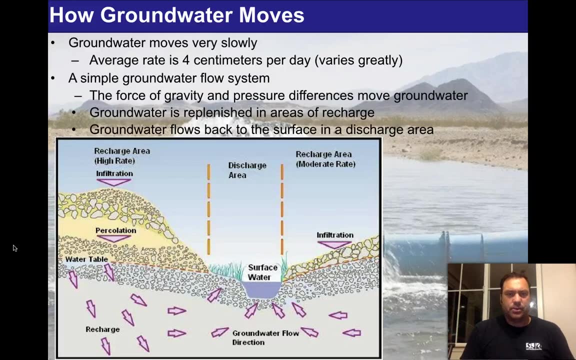 karst- well, not karst topography, but it's created in karst topography systems. where the limestone is completely dissolved away, It's obviously able to freely transmit groundwater On average, though I mean we need to be kind of aware of how. 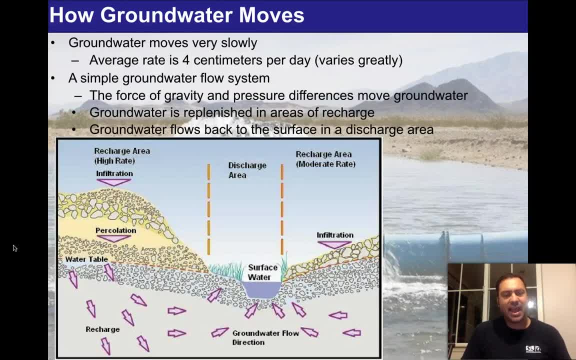 these things operate. There's a large amount of variety, but on average, the average rate is four centimeters per day. That's about that big right, Not much So. water underground flows slowly, A simple groundwater flow system, basically the force of gravity and 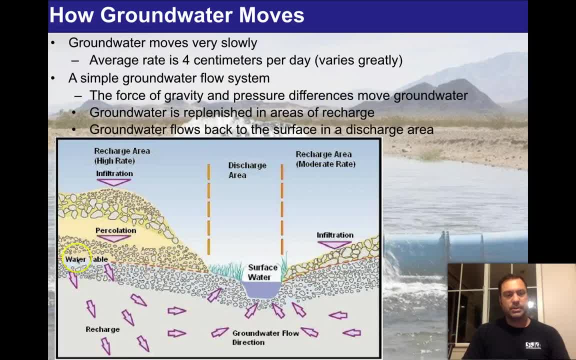 pressure differences move the groundwater right. So here's the water table. This is sitting higher and therefore has more gravitational potential. This is sitting lower, has a lower gravitational potential, So the water will flow from high to low. That's basically what we're seeing here. So here. 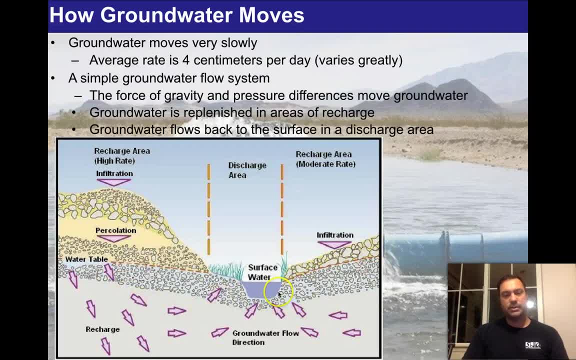 are the arrows you see going from high to low. Here again from high to low, And so we see a surface water and a gaining stream here. So this becomes the discharge area, In other words where the water actually flows out. So groundwater is replenished in areas of recharge. So here we see a recharge. 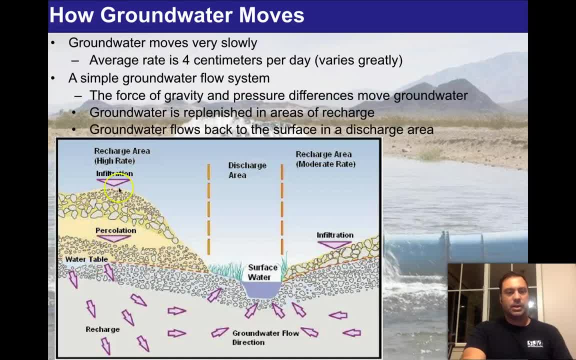 area. So here's our vato zone. We have percolation, The water infiltrates in from up on top of this ridge and then infiltrates here And eventually it discharges into the stream. right, We're going to go ahead and say the stream is. 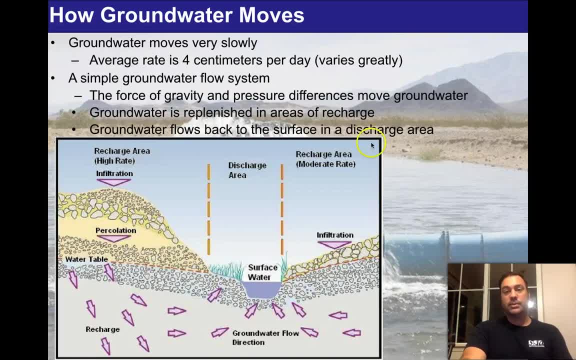 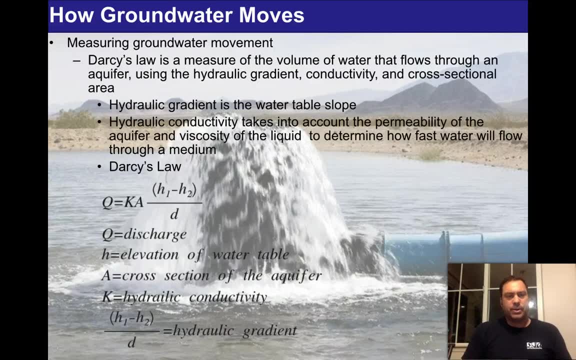 a gaining stream system, The groundwater flows back to the surface in a discharge area. Pretty straightforward. How do we go about measuring groundwater movement? Right, there's different ways that we can do it. You can throw a die in the water. We can see how fast it moves. But the problem is, is that underground you? 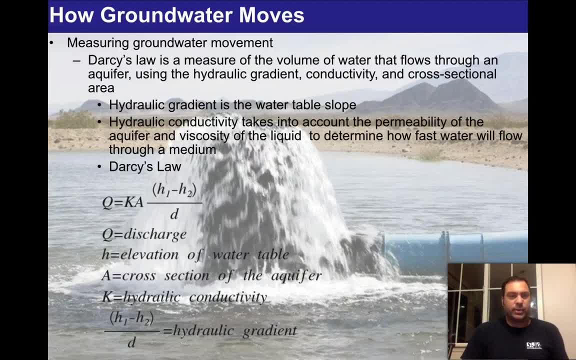 can't always track these things very easily. Fortunately, there's a really interesting relationship that exists in water. that was discovered by a guy named Darcy, And Darcy came up with something called Darcy's Law. He was looking at how water flows through an aquifer- different kinds of aquifers- And he came up with a. 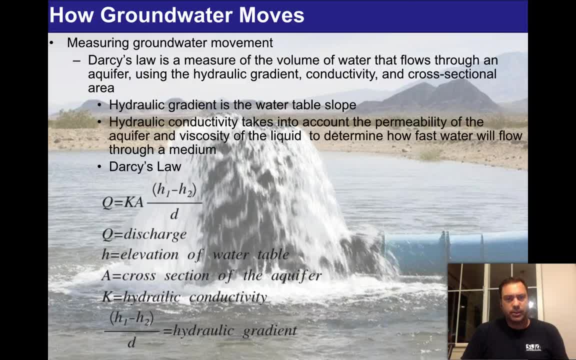 really cool mathematical relationship, So I just want to show you a little bit of that. I want to introduce it really quickly. So Darcy's Law is a measure of the volume of water that flows through an aquifer using the hydraulic gradient. We'll come. 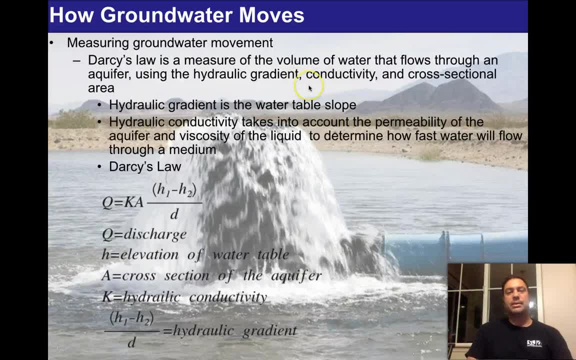 to what that is here in a minute: The conductivity. So the conductivity is the porosity and the transmissivity, In other words, the ability for water to flow through And cross-sectional area right, Which is say the cross-sectional area of. 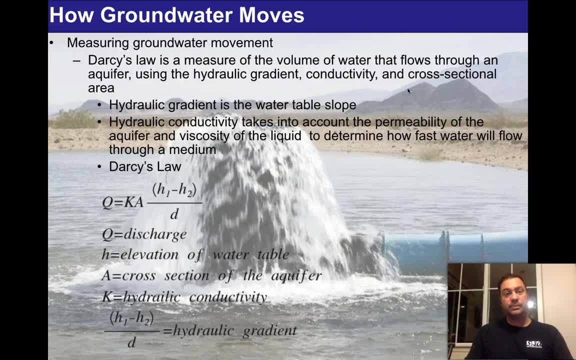 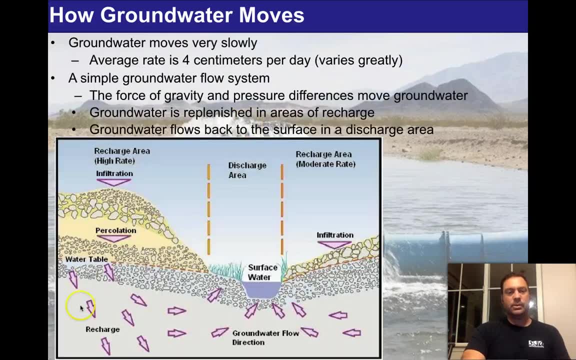 the aquifer or the aquifer section that we have an interest in. So, basically, the hydraulic gradient is the water table slope. Okay, We saw this here. Here's the high, here's the low, and this angle right here is the slope that. 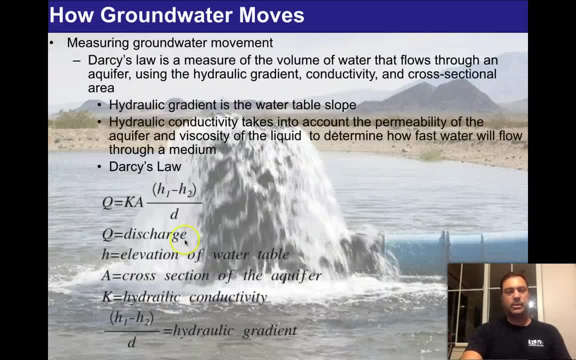 it's talking about. We'll come back to this and how we measure this in a moment. Hydraulic conductivity takes into account the permeability of the aquifer and viscosity of the fluid. This is another thing I haven't brought up yet. Water actually has some viscosity, In other words, a resistance to flow. We 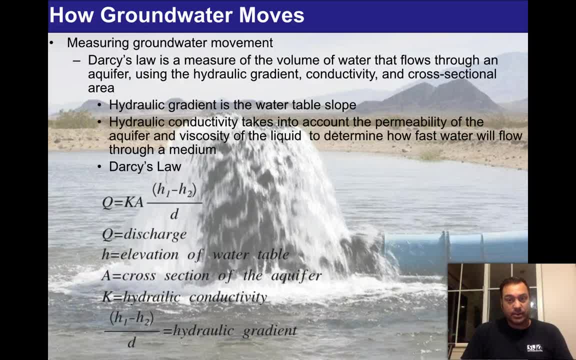 talked about viscosity when we were talking about different kinds of lavas Way at the beginning of the class. So, anyways, this is a resistance to flow, It turns out. water has a certain level of viscosity. The colder it is, the higher the viscosity. The hotter it is, the lower the viscosity. Okay, So the viscosity of 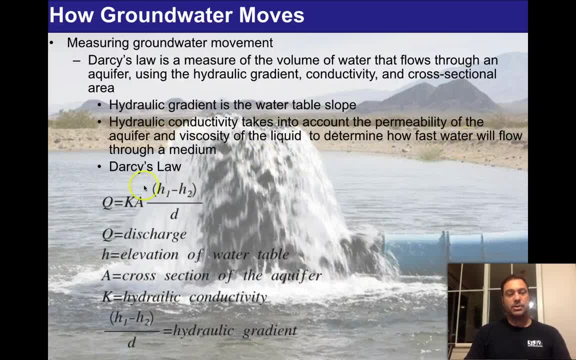 the liquid to determine how fast water will flow through a medium. So here's Darcy's Law. Okay, So it's this relationship. here, Q equals Ka over parentheses, H1 minus H2 over D. What does all this mean? Just simply is this. 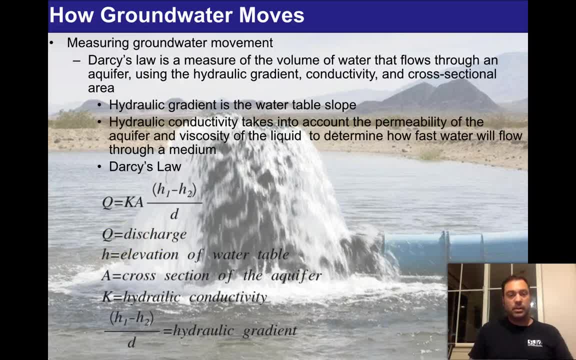 Q is the discharge. It's the amount of water, H is the elevation of the water table. We have two different points right. We have one at one point maybe it's the top of the stream and the other one is maybe at the top of the well And we can. 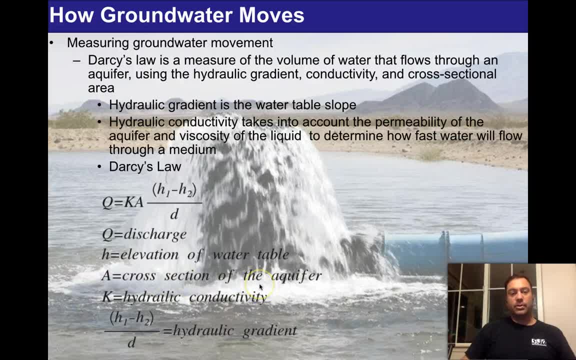 measure these two things. We can look at the cross-section of the aquifer, In other words, the area that we care about of the aquifer. We can figure out the hydraulic conductivity. Usually this is given to you by a scientist that has 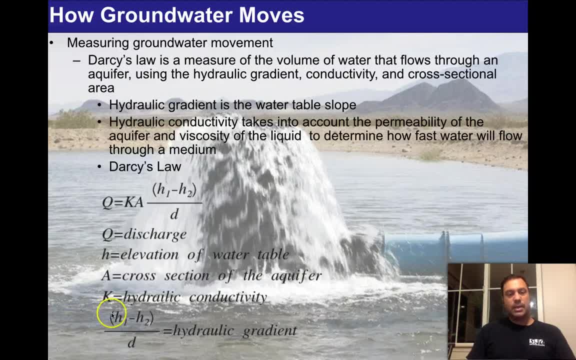 figured this out and solved this And we can calculate the hydraulic gradient. Now, hydraulic gradient is pretty straightforward. Let's go ahead and introduce this right here. So this whole thing right here is just this section. We're really just multiplying three numbers: K, A and then 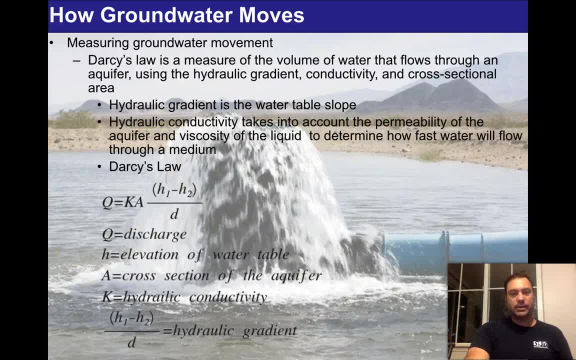 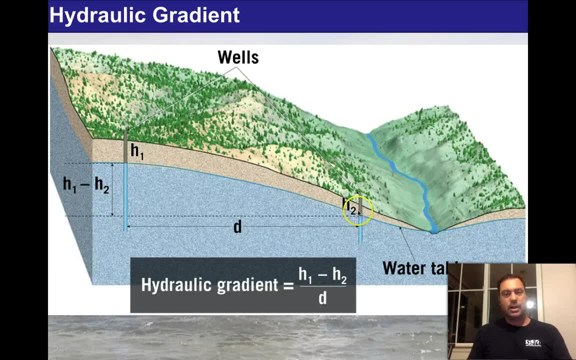 whatever this hydraulic gradient is. So this hydraulic gradient is just simply this: right Here we have height one, So some height up in the mountain. Here's another height. The water table is this blue section right here, beta zone. So here we have an H1 and H2. And we can just simply take the difference between. 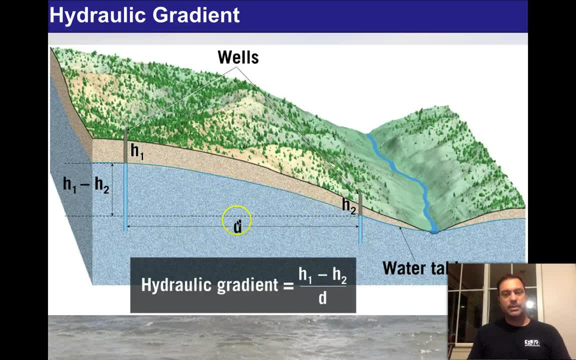 the two Right, H1 minus H2, divided by the distance. That gives us the gradient that we need Right. The cool thing is we don't really need to worry about units so much, because this would be in meters, that would be in meters and this is gonna be. 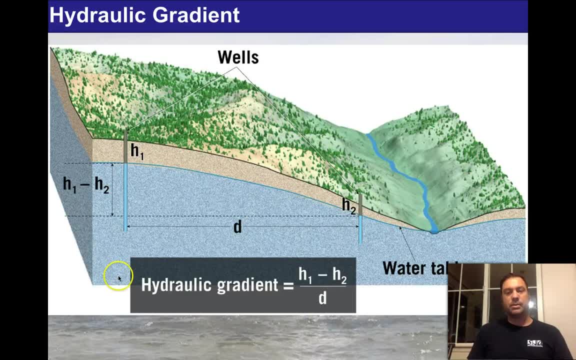 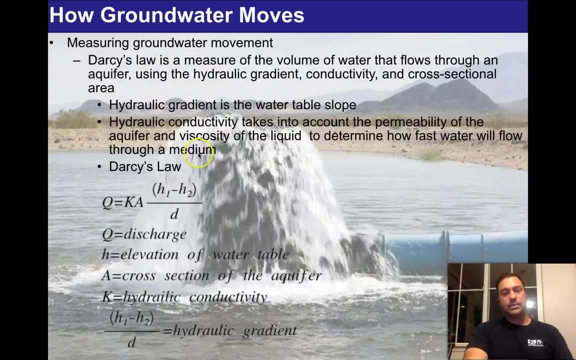 in meters. It winds up dividing out and it just winds up becoming a dimensionless number. Makes calculation very, very easy. Okay, So that winds up becoming a single number. That single number is just multiplied by K and A, which you can measure right off of the diagram or it's just given to you by a. 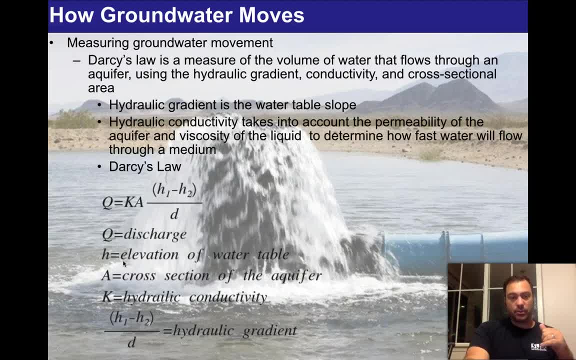 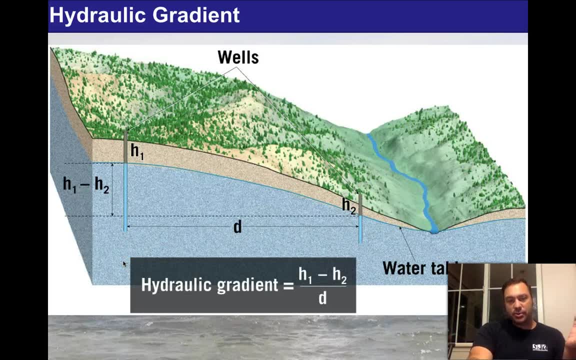 by whoever's interested in that particular aquifer. Cool, By the way. this is extremely powerful because it tells us how much water is being fed into a certain area at any given time. If we know these things, we can figure out how fast the water is moving. We could figure out, you know, what direction it's going. 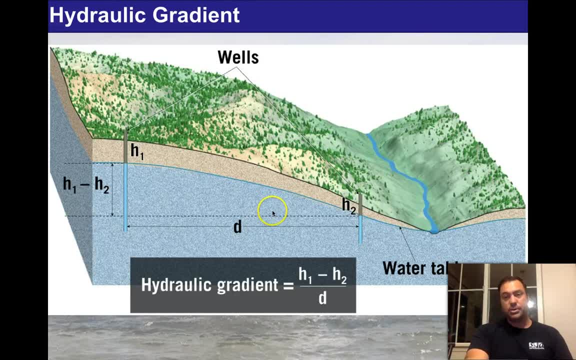 But, even more importantly, we can figure out the volume, the total discharge, how much water we can pump out of there and know that the water will not diminish, It won't go away. Right, This is really important. We also need to talk about different ways that groundwater moves. So when we 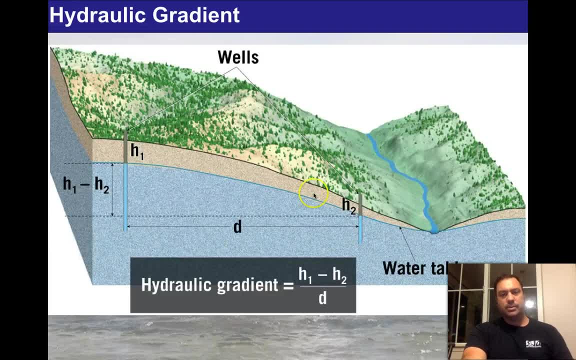 talked about this previously. let me go back to this. Notice that this diagram here kind of implies that everything below this water table is just really, really boring. Right, It's like almost like an underground lake, filling all the little pore spaces. It doesn't really work like that in nature. It really looks. 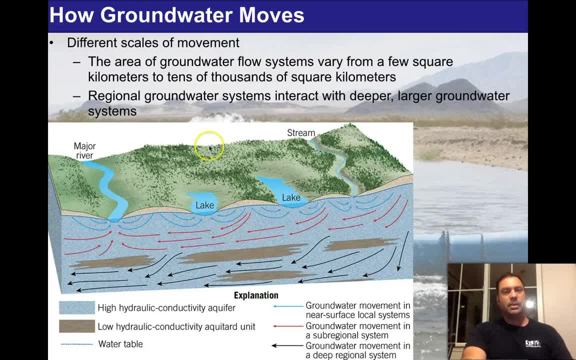 more like this And we have different scales of motion, So the area of groundwater flow systems vary from a few square kilometers to tens of thousands of square kilometers. Right We have regional groundwater systems that interact with deeper, larger groundwater systems, So here we have a lake and a 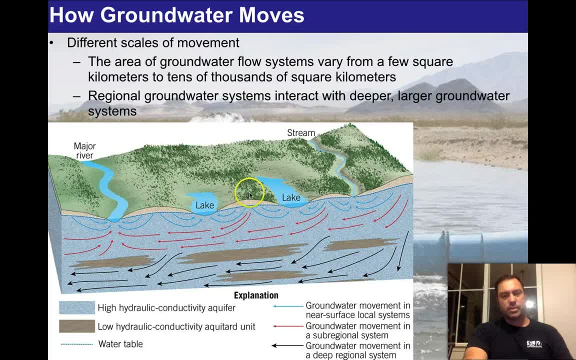 leather lake and some streams And notice that the wave of water is actually coming from areas of infiltration and it's distributing into the lakes Right The same thing, into the streams. maybe a major river, But then some of it actually percolates down below and it's not interacting with the topography. 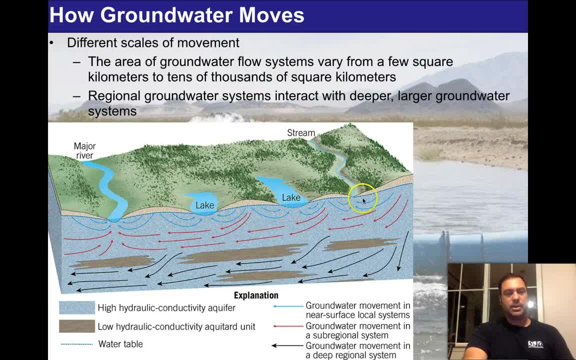 Notice this, by the way, the subdued mirroring of the topography up above. But this red zone is not really responding very strongly to it, except for right here at this major river. This major river does have a significant effect on the overall flow of water, And then notice that there's some black lines. 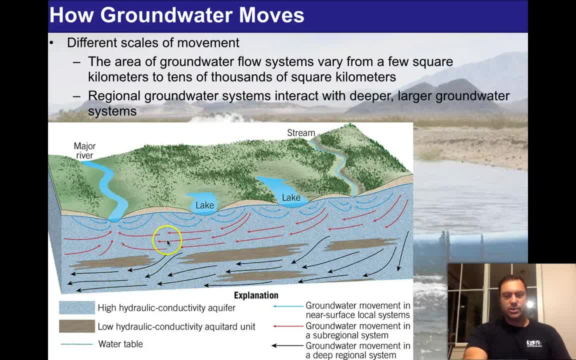 down below. This is going to be a deep regional system And a lot of what's going on down here is not being affected by what's up here. There's water coming in but maybe not a whole lot coming out, And the reason why this is happening is 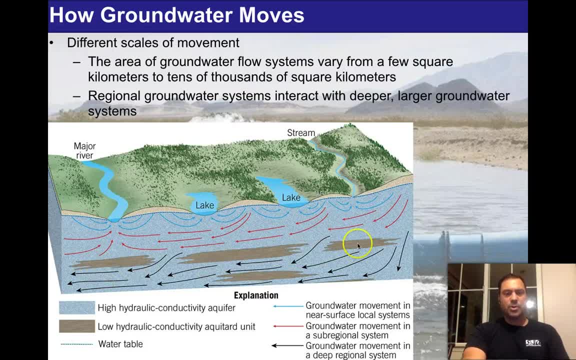 these brown zones right here are basically aquitards, And what it does? it separates what's going on up here, on the top, from what's going on down below, And so we have a layered system. There's structure down there, And this is really. 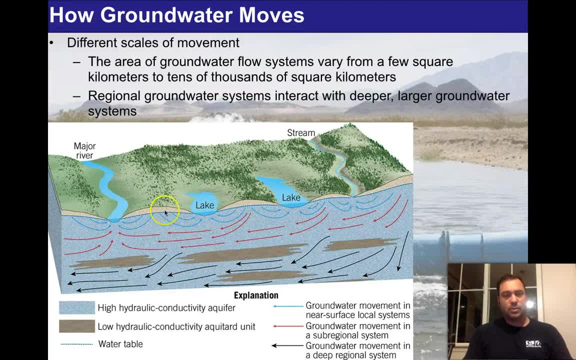 important If we want to know, if we're drilling and interested in water that's maybe shallow versus medium or even very deep, we need to know the overall system and how it's behaving. So our relationship, our Darcy's Law might give. 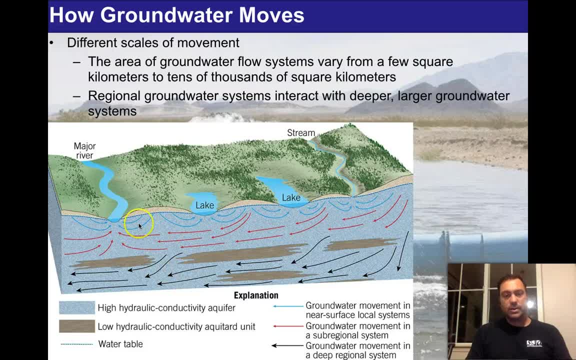 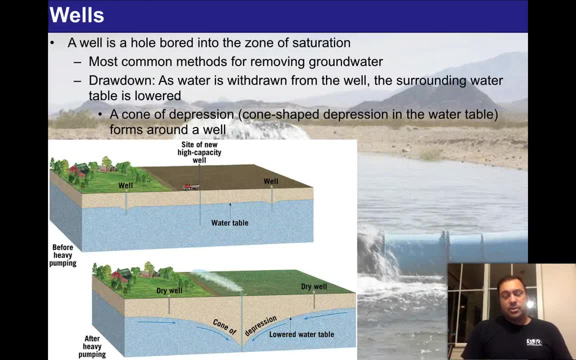 us different answers for here and here and here We need to know the parameters so we can get it right. So the way that we do this is we basically do it with water wells, right? So a well is just simply a hole that is bored into the 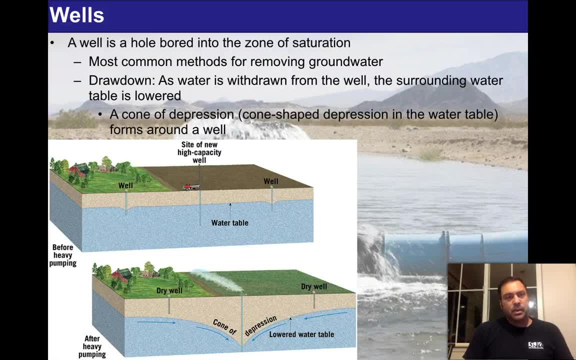 zone of saturation right up, right down into the aquifer. The most common methods for removing water is almost always a well. There's other ways that you can do it, but it's far and away the most common. Now, one of the consequences of drilling a 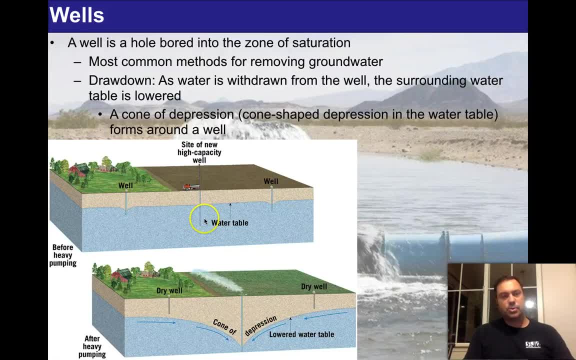 well and pumping the water out is that you get something called drawdown. So here we got this, well, it's been installed and we start using it to irrigate this field. And what it does? it draws down the water table. Now, what does? 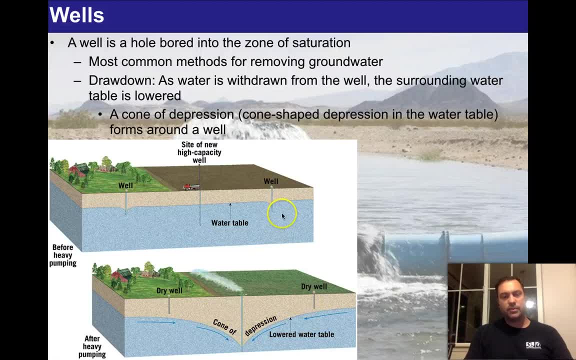 this do? What it does is it forces the water that might not be moving very fast to suddenly move towards your well, right? So this well and this well starts drawing all this down And there's a couple of effects, right? So in our 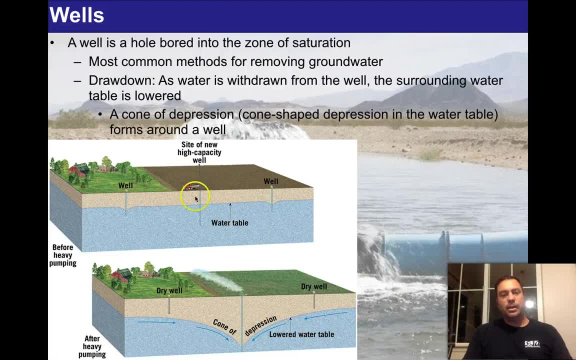 original document. this or, I'm sorry, in our original part. up here we have. the well is being installed. the water table is nice and flat. We have a little bit of drawdown around this well. It's owned by this property owner. This property owner, which is the same here, is. 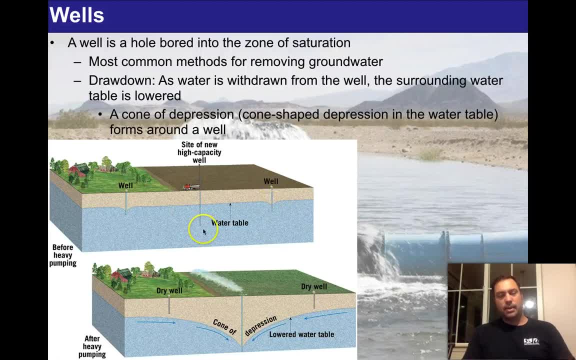 drawing down And he just basically says: I'm gonna dig deeper and I'm gonna drill harder or pump harder on that aquifer and use it to irrigate my field, And what that does is it drops the cone of depression. but now this well, no longer. 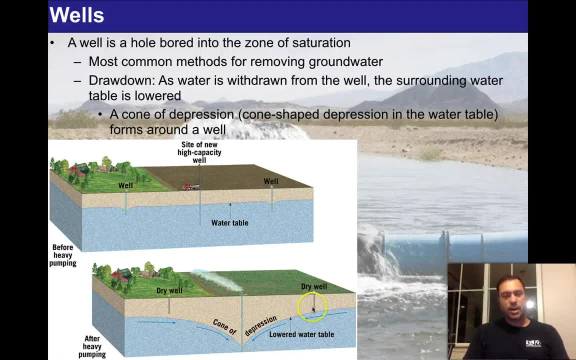 is in the zone of saturations. This, neither is this one, So these both go dry, which of course doesn't make this person very happy, And you get this very large cone of depression from the heavy pumping or usage by this agricultural well. So this is, of course, something that is very 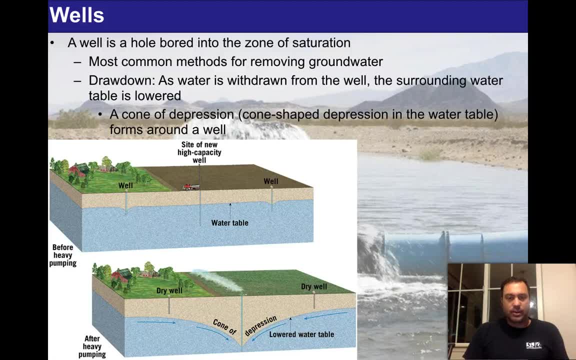 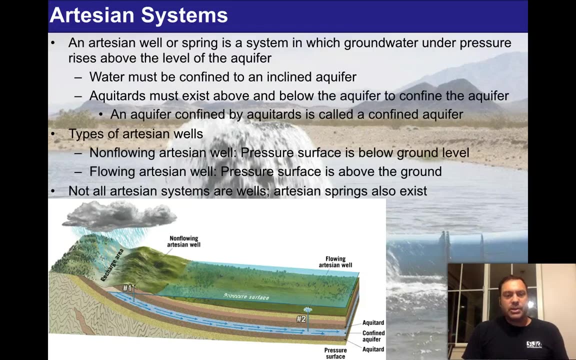 closely monitored by state authorities nationwide and usually worldwide. You know, in most developed countries maintenance and understanding of where the water table is is watched very carefully by municipal authorities. There's another kind of system that I wanted to bring about really quickly as we're kind of going through. You might be familiar with the situation where water 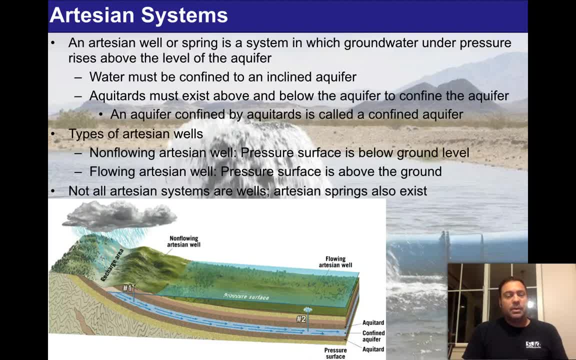 just kind of flows out of the ground. We call those a spring. How do those form? What is that? Well, let's talk about that. So an artesian well, this is a well that flows out of the ground on its own. So, in other words, you put a tube in the ground. 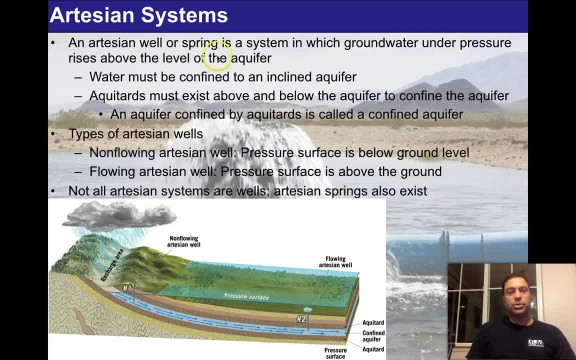 and the water just comes right out on its own. Or spring is a system in which groundwater under pressure, which is say under natural pressure, rises above the level of the aquifer. How does that happen? So water must be confined to an inclined aquifer. So in other words, we have water with an aquitard above it, and 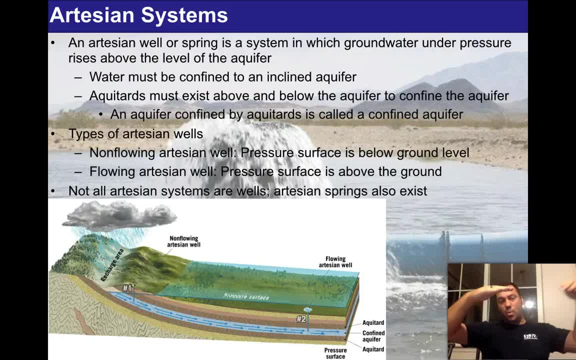 an aquitard below it right And there's a nice aquifer in the middle. The water's trapped in there. It can't get out, It can't move above, It can't move down. It's stuck inside of this aquifer for better or for worse. okay, An aquifer confined. 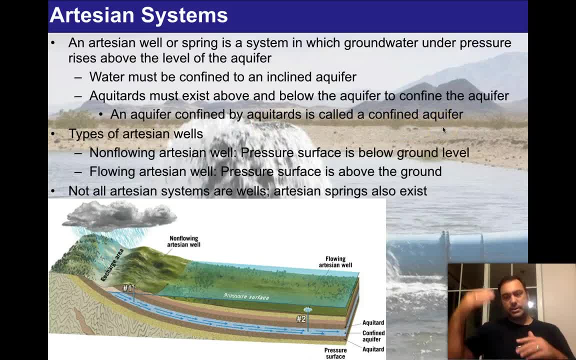 by aquitards is called a confined aquifer right, So it's basically sandwiched by two aquitards. The water cannot get out. So there are different kinds of artesian wells. There are non-flowing artesian wells, where the 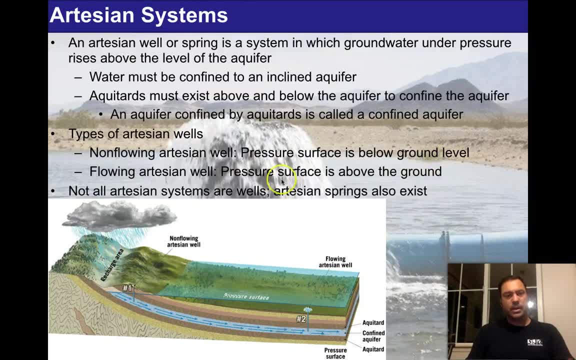 pressure surface is below ground water or at ground level. But a flowing artesian well is where the pressure surface is above the ground. In other words, here's a recharge area. here The water is on the ground, The pressure surface is above the ground. 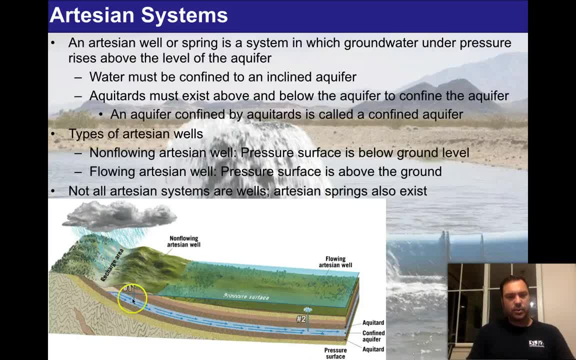 The water is in here And we could even put in a well. There's a non-flowing well. that's right here, because it's sticking above the pressure surface, And the pressure surface extends in this case out into the open area and even above. 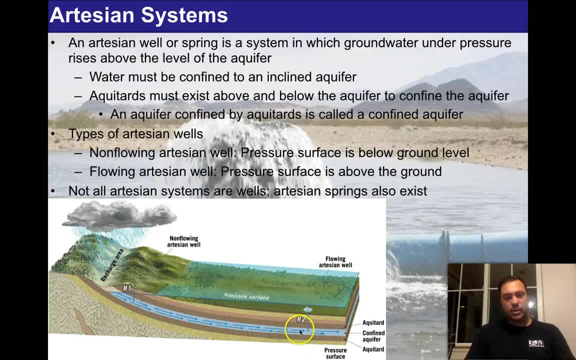 the land. In other words, if I stuck a well here, the water would want to rise up to the top of that pressure surface and hold its level there right. It's kind of like if I have a hose right. Imagine I have a clear hose, which I wish I had, and I 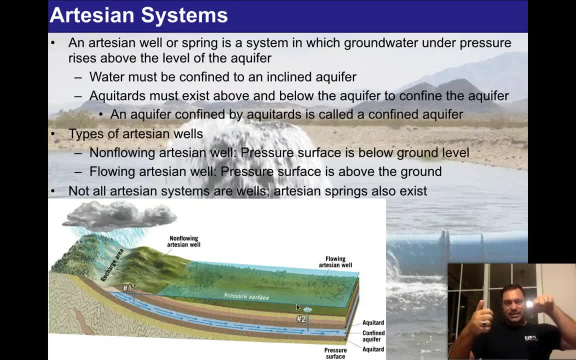 don't, And I put water in one side, it's going to fill up to the exact same level on the other side of that hose. on both sides It's going to even out. That's basically what's happening here. You're dumping water here. 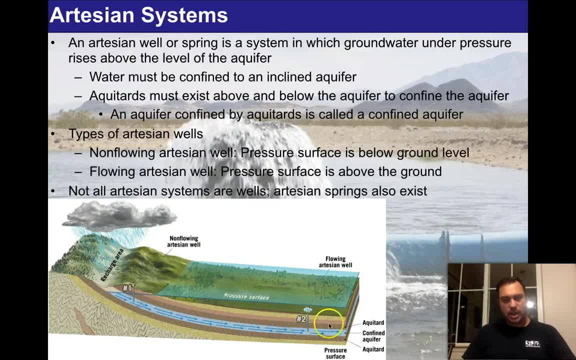 and it's trying to even itself out somewhere along here. But look, this aquitard is not allowing the water to come up, It's confining it. So, as a consequence, there's a natural pressure built up, And if I stuck a well in there, the water would come out on its own. 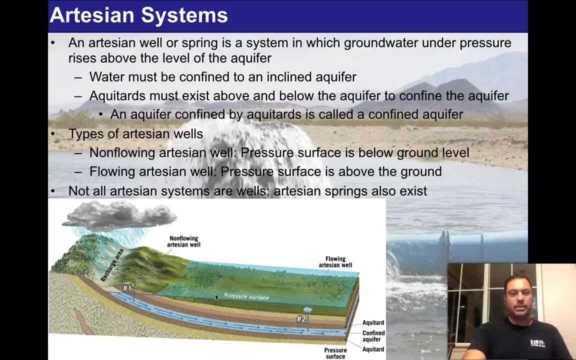 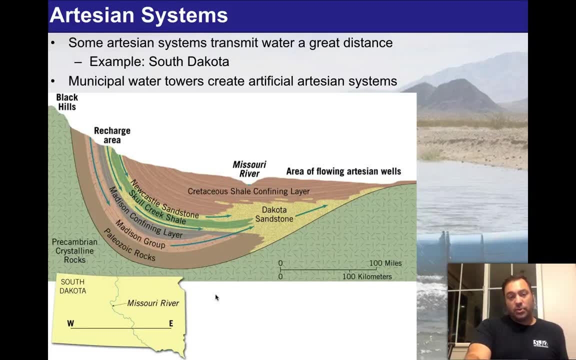 I wouldn't even need to pump it out, It would come out on its own. These are really, really cool And, by the way, these don't have to be local things, right? In this case, this is one where we just see it coming out of the mountains and showing up here in the valley. But these 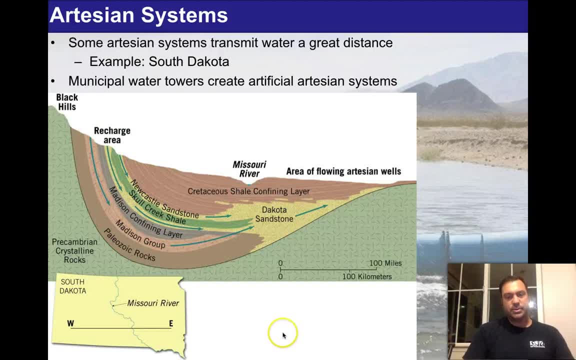 could be over very long distances, hundreds and hundreds of miles. In this case we see artesian systems that transmit groundwater all the way into South Dakota. right Municipal water towers create the same artificial. We'll go into that in a minute, But here's. 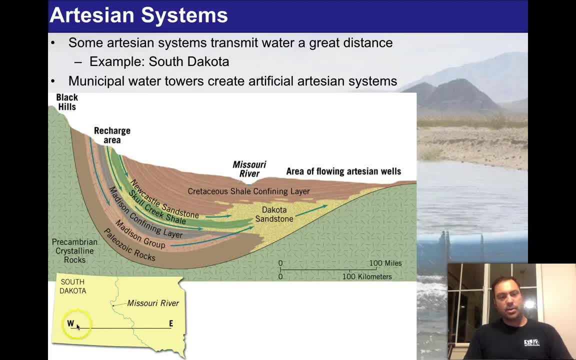 the recharge area. This is, by the way, going across from South Dakota, and the discharge over the Over here is on the other side of South Dakota, in the east. Basically, it's coming out of the Black Hills, It's getting into the Madison Group, It's getting into the Newcastle Sandstone. 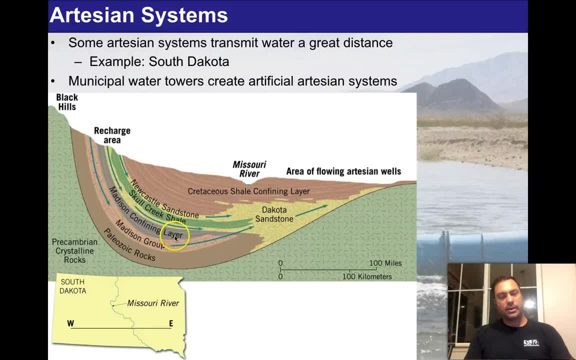 And it's confined by the Madison Confining Layer, which is an aquitard- The Cretaceous Shale, which is also an aquitard. That water, basically, is piling up over here and putting pressure on water that's already in the Dakota Sandstone. So what do we see here? There's 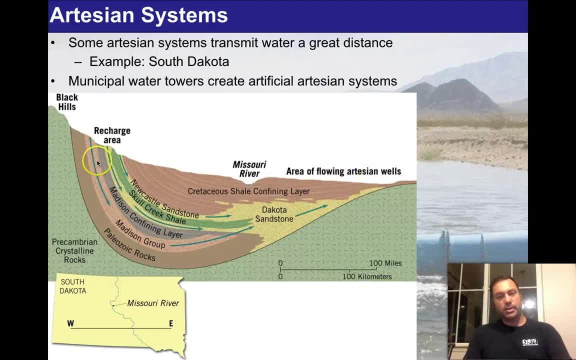 flowing artesian wells all over the place over here, as the water that is over here is putting pressure over here, And basically municipal water towers are artificial versions of this, where we pump the water up high and that puts pressure down into the pipe. 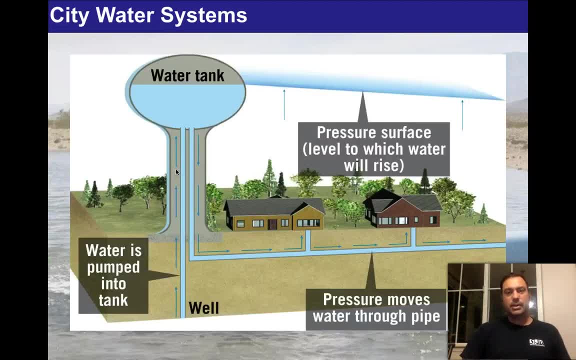 so that when you turn on your faucet, the water comes out just like this right. So we put the water into the tank. That creates a- I'm sorry- a pressure surface. I use the word potentiometric frequently. That's how us geologists refer to the surface That's. 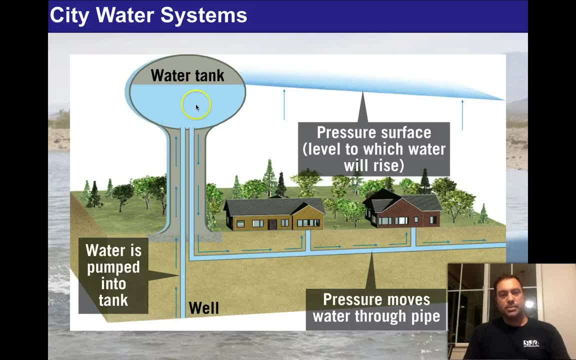 a pressure surface And this water tank Basically it's a pressure surface And this water tank basically is putting a bunch of pressure down, gravitational pressure, and it basically feeds the water not only to the houses but it gives some pressure to that water so that 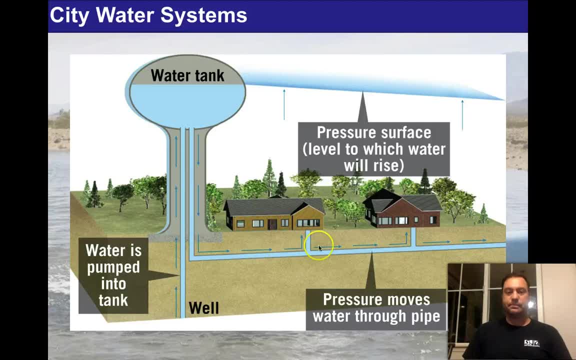 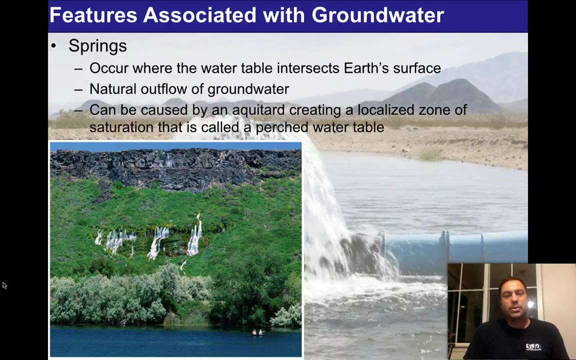 when you open up the faucet, the water comes out and into your drain- Okay, it's the same thing here- And then it flows right out through your drain system. Okay. A couple other things I want to bring up here, mainly springs, right, Springs occur where the water table intersects. 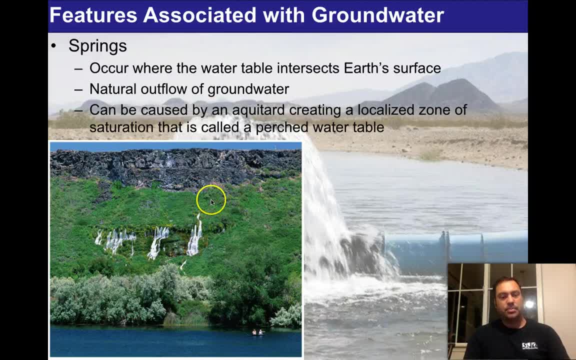 Earth's surface. So here we see a water table, probably a relatively confined one, but there's a recharge area up above And basically the Earth's surface here has been broken apart, exposing, basically cutting the aquifer, so the water is just flowing right out, right. So this 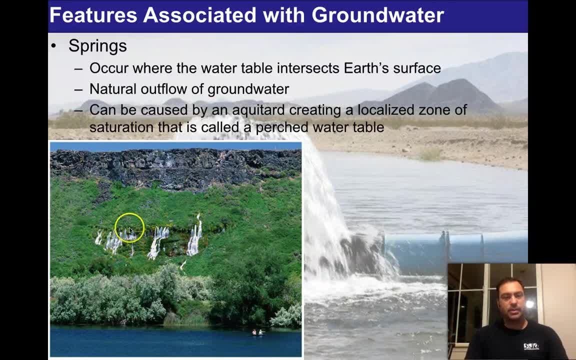 is almost like an underground river. Notice there's no water up here. It's coming right out of the rock right here And it's a natural outflow of groundwater And it can be caused by an aquitard, creating a localized zone of saturation called a perched water tail In. 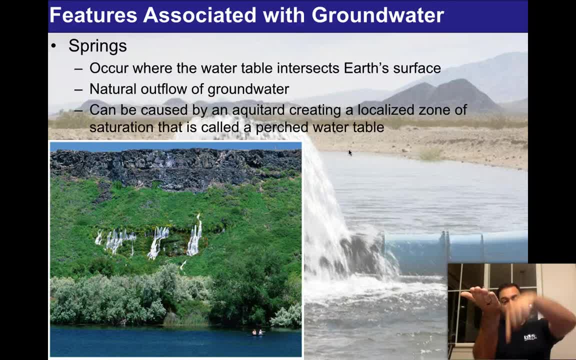 other words, a zone where the water is not allowed to fall all the way down into the deep aquifer. It's being held aloft or perched up onto a higher level, And this is, in fact, exactly what this is. The potentiometric surface is right down here at the lake. The water 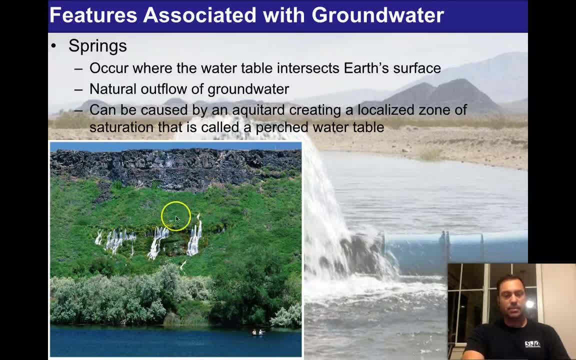 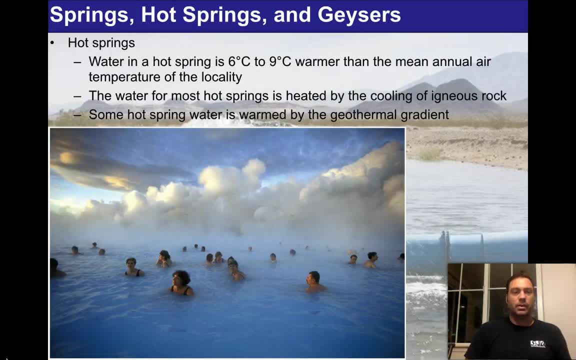 and underneath theücht is this beautiful waterfall, Very, very cool. Okay, Hot springs. right, We are not always dealing with just cold water falling out of the sky and running all over the place. We've got these things called hot springs, You know. 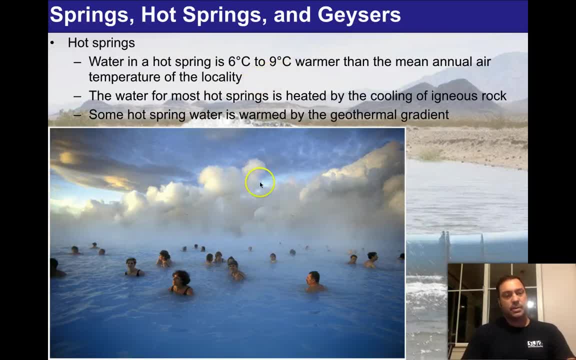 this is where the water can be 6 to 9 degrees warmer and Celsius right Degrees Celsius warmer Than the mean annual temperature of the locality. So this is a situation in Israel where people are enjoying a nice hot spring. I think it's adjacent to the Dead Sea, The 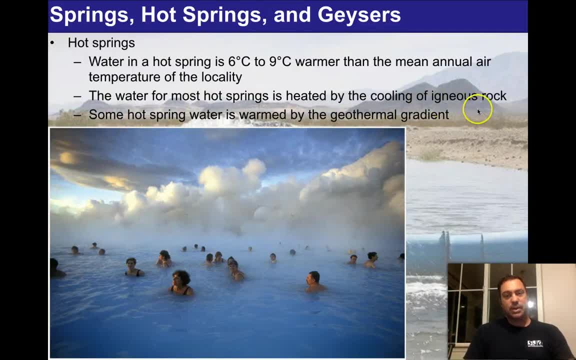 water fromnea most hot springs is heated by the cooling of igneous rock- We've talked about hot springs before- And some hot spring water is warmed by the geothermal gradient. In other words, the water is going through the, you know, for example, 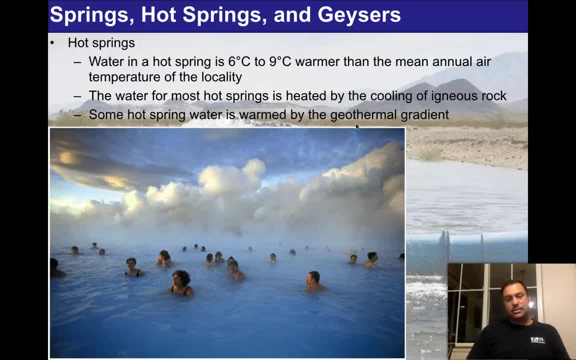 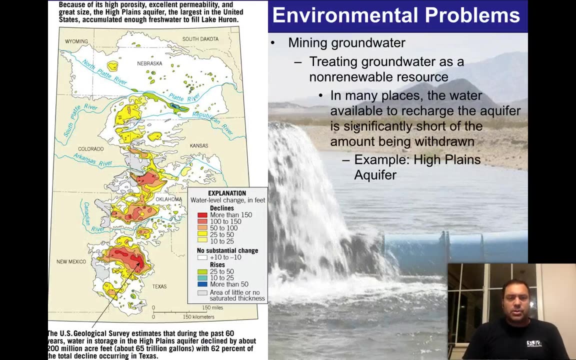 from the Black Hills. it warms up as it, as it's rocked down into the earth. The earth warms it up. When it finally comes up, it comes up a few degrees warmer And it could be quite comfortable, So that the fact that this groundwater is so 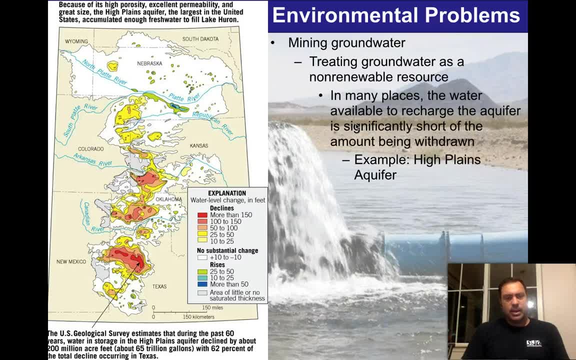 useful and is so available has brought some problems right, Some environmental problems. We tend to mine groundwater. We need to, and I use this word mining in an interesting way. we tend to think of water as being a renewable resource, And in many ways it is, But we really need to think about 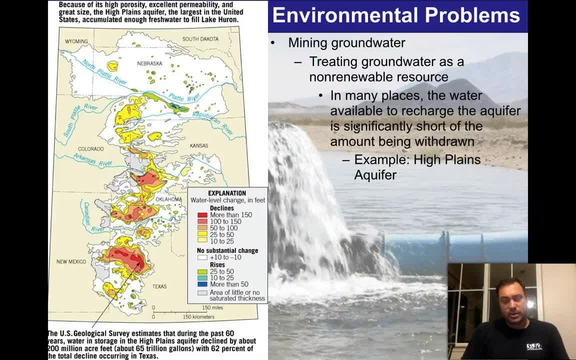 renewable resources as being on the surface in terms of water, Rivers tend to be renewable. Oceans can be somewhat renewable you as long as you don't completely destroy them with pollutants. But groundwater is a little different. Remember, the flow rate on average in an aquifer is only 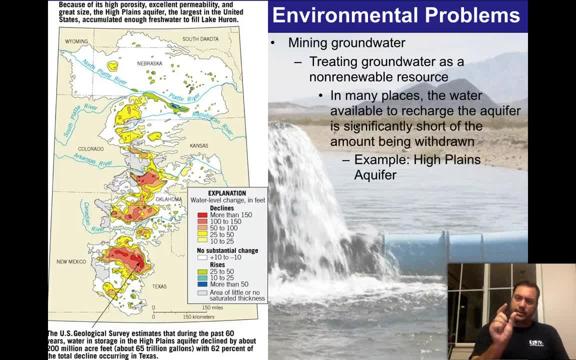 about four centimeters per day. That's quite slow, You know. this is about like this on average worldwide. So we need to think of groundwater as possibly being a non-renewable resource, at least on human timescales. So in many places the water 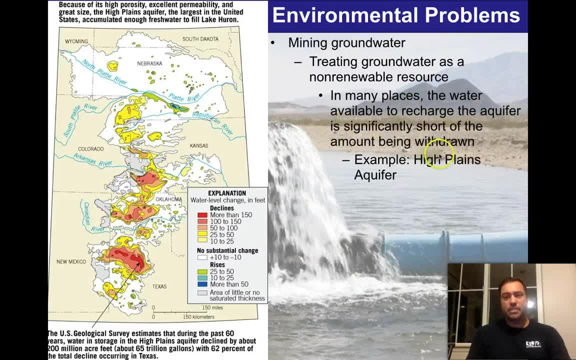 available to reach our geographer is significantly short of the amount being withdrawn. In other words, there's a huge demand for water, But maybe nature isn't putting the water into the system as much. In other words, we have ancient rainwater that is stored in these aquifers and we're pumping that out. 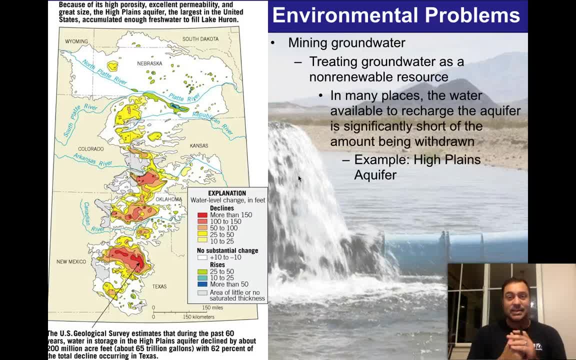 faster than the earth can replenish that And in that sense, it begins to act like a non-renewable resource. Well, some of the places we can see this is we can look at water level changes right, And here in this map, here this is the High. 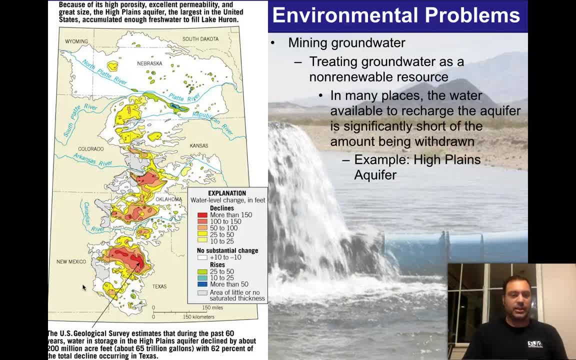 Plains Aquifer, which is in the Midwest. It feeds a lot of the agricultural zones of western Oklahoma, Kansas and Nebraska cornfields in northwest Texas. And what do we see here? We see that up here in northwest Texas, this red zone, 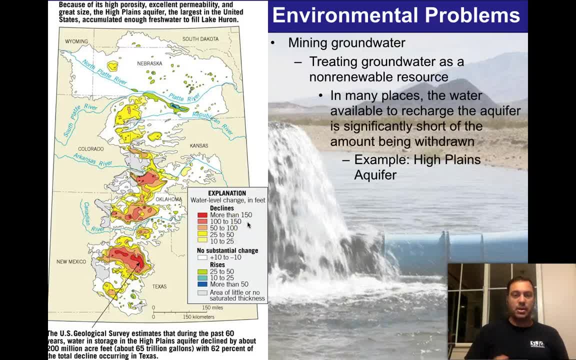 here is an area of more than 150 feet of drawdown on that water level, In other words, a very large drawdown. We see another drawdown here in. well, this is again still in north Texas and Oklahoma and, of course, in southwest Kansas we see. 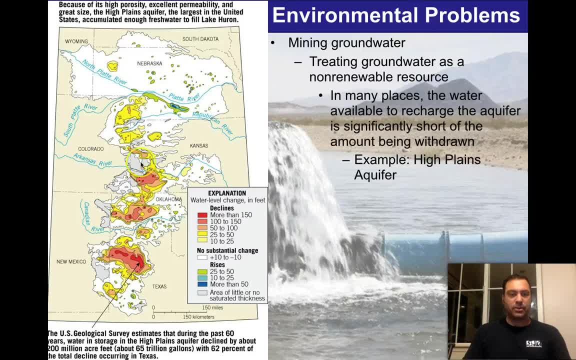 the same thing: Incredible amount of rainwater. We see that the water level has dropped considerably. This is a tremendous amount of drawdown and it's essentially a threat to the aquifer itself. Another environmental problem is subsidence: right When you have water in the ground. 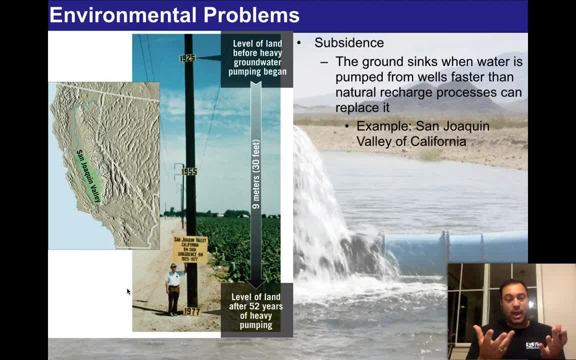 it basically is part of that earth and it's making up some of the volume that's holding the earth up right. So when you pump the water out, what happens? It's not going to be able to pump the water out. It's not going to be able to. 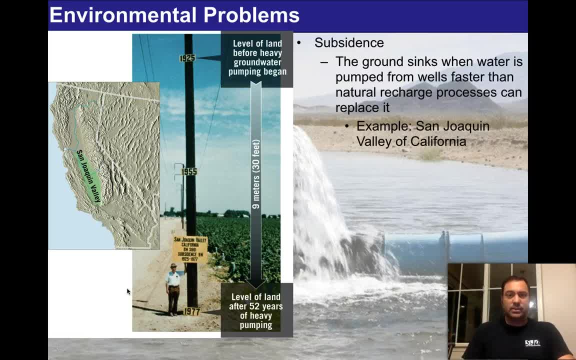 pump the water out. It's not going to be able to pump the water out. It's going to sink. What does the ground tend to do? It sinks. This is the San Joaquin Valley of California in 1925. This is where the land was in 1925. This is where it was in. 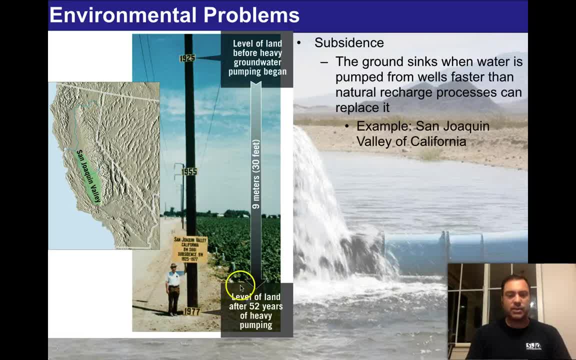 1955, and this is where it was in 1977. This is 52 years of heavy water pumping. The San Joaquin Valley is an area of extreme agricultural water usage, So it's dropped 30 feet since, from 1925 to 1977.. Unfortunately, I don't think it's going to. 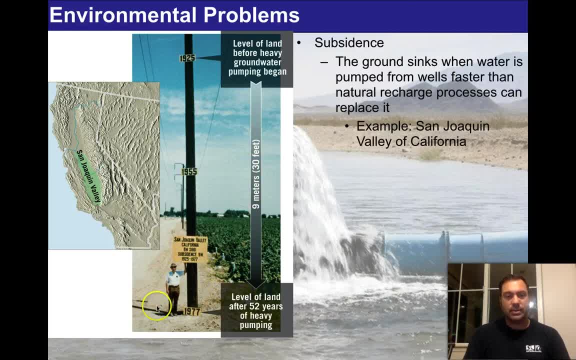 have any data since then, but this is an interesting picture, right? This is the amount of water that has been pumped out of the earth in this area. Now can we recharge it and push it back up? Possibly, I don't know the science. 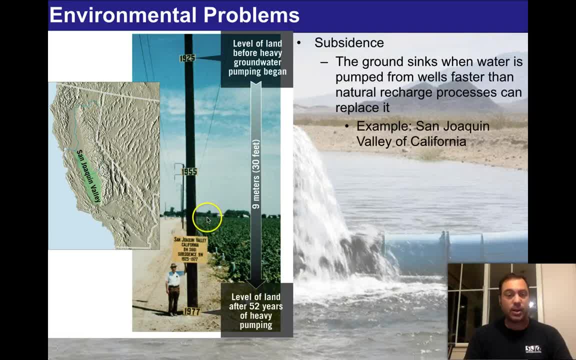 specific to the San Joaquin Valley, but it can create some interesting prospects of what we call groundwater recharge projects. So anyways, California is a state that is subject to extreme levels of drought. Freshwater water systems can be threatened by a couple of rainless years, or relatively. 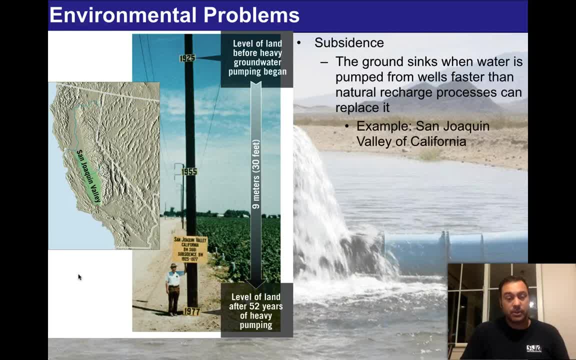 low precipitation years. So the politics in these areas can be quite dicey sometimes, But anyways you get the idea. Pump the water out and the ground starts to drop. This also, by the way, happens in a lot of oil fields too. 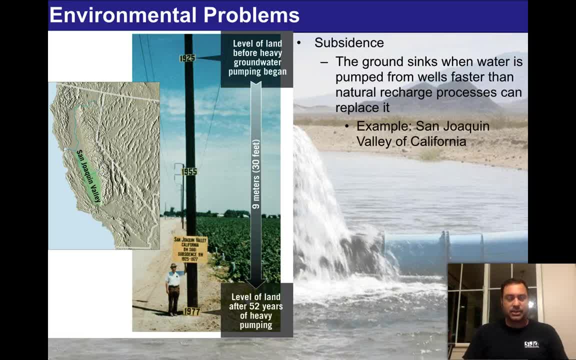 But a lot of the oil companies, to maintain these subsidence, will actually pump out oil and then replace it with seawater to try to maintain the balance, to keep the sea out of the water Or, I'm sorry, to keep the land level over time. 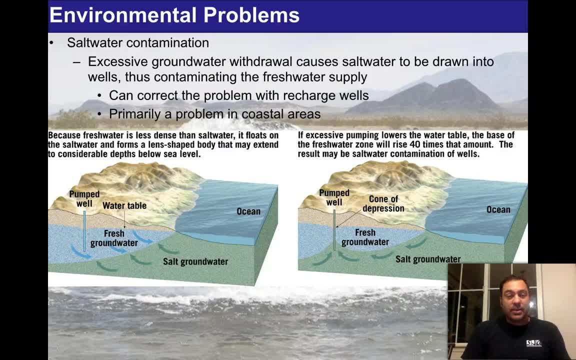 Okay, another consequence: Wow, there's all kinds of different things that we need to be careful of: Saltwater contamination right Along coastlines. we can start drawing down the groundwater, but it also has the effect of drawing up saltwater. Now, the problem with saltwater in the ocean is that saltwater 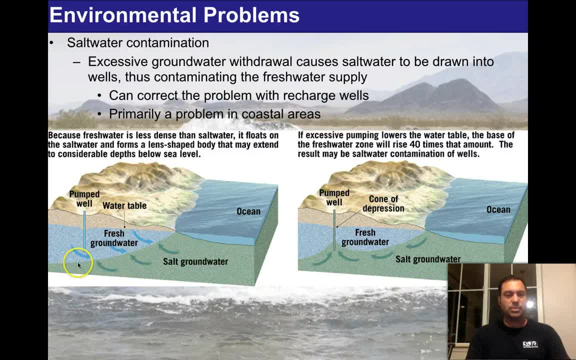 will actually form in this relationship. we see here, it'll actually proceed underneath the water table, And the reason why this happens is that salt groundwater from the ocean, fed by the ocean, is denser, So it sits below the freshwater along the coast. So if we're pumping along the coast, we have to be 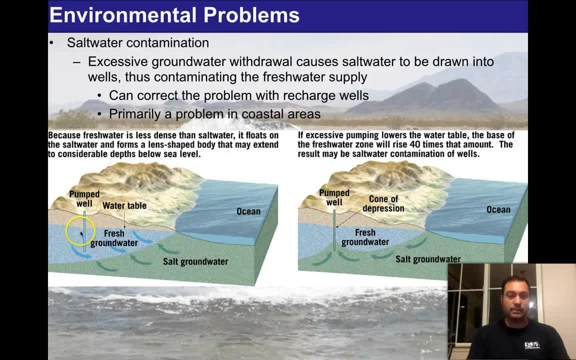 careful of the fact that we may create a cone of depression up on top, But we can also create a cone of depression down below as well and start sucking up groundwater. The moment we do that, we basically destroy the well right, The. 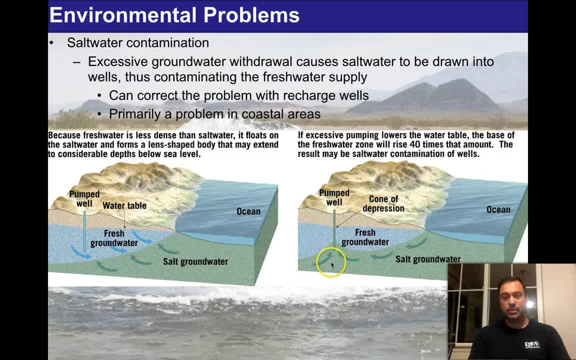 well is no longer useful unless we carry on pumping the saltwater down the coast. So that's the reason why we care about getting salt groundwater, But what that does is it draws the water up and it encourages more saltwater from the ocean to come into the area beneath the fresh groundwater aquifer. 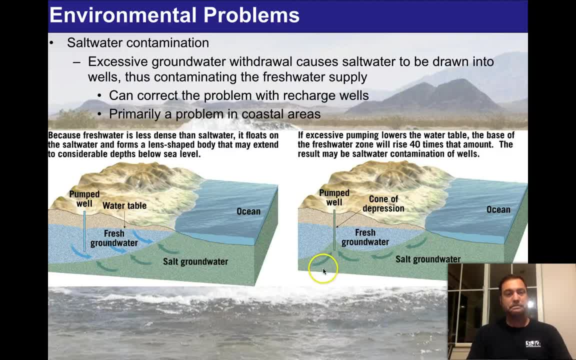 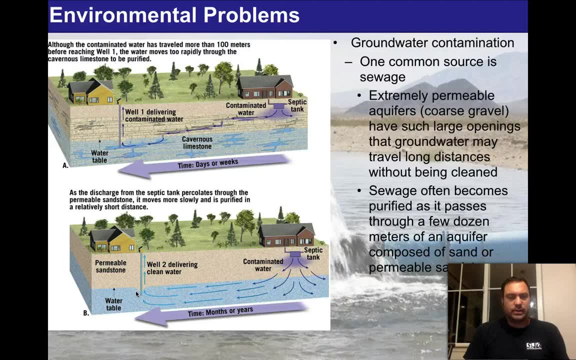 These are generally not good things. Another environmental problem is sewage right. Not just sewage, but septic tanks in particular. So in some ways it's a good thing to have a septic tank, because you don't need these complicated and leaky system sewage systems that can cause all kinds of problems. but on the 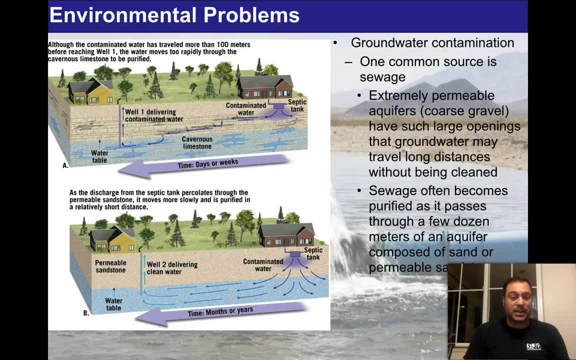 other hand, if it's not managed properly, it can make people sick. it can actually destroy an aquifer. so basically, when wherever they install a septic tank, so in this case, here we might have cavernous limestone down below and here we got a. well, this guy is actually drinking the water out of the aquifer. 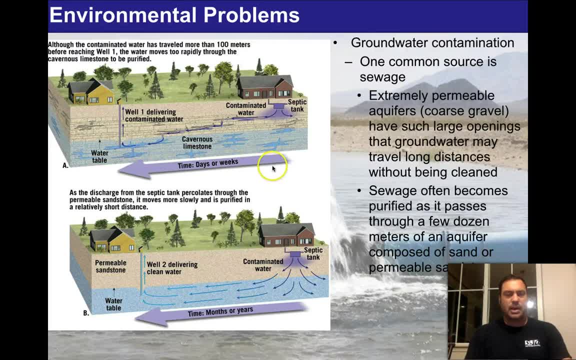 and this guy's got a septic tank right and the amount of time to go from his house to his house may be days or weeks, right, because remember four centimeters per day. we do Darcy's law and we figure out this information. if we were. 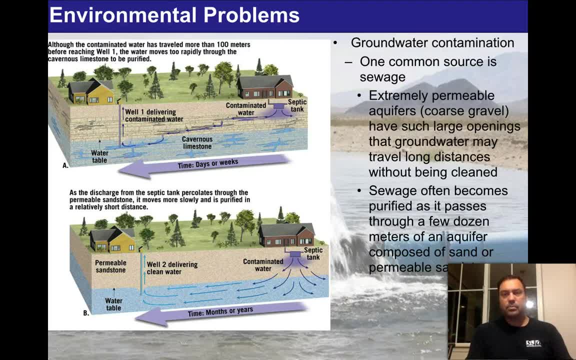 engineers wanting to know if these houses would be safe. so extremely permeable aquifers such as coarse gravel or cavernous limestone have such large openings that groundwater may travel long distances without being clean. so one of the things that tends to happen is you flush the water out of the aquifer and then you flush the water out of the 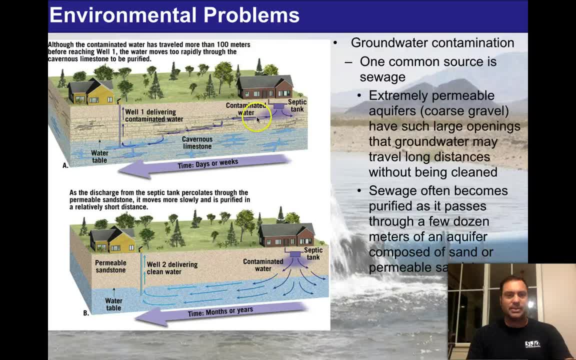 toilet goes into the septic tank, and the contaminated water as it's moving through the system tends to clean itself, or what we call attenuate. it purifies. okay, sewage often becomes purified as it passes through a few dozen meters of an aquifer composed of sand or permeable sandstone. there's there's all kinds of 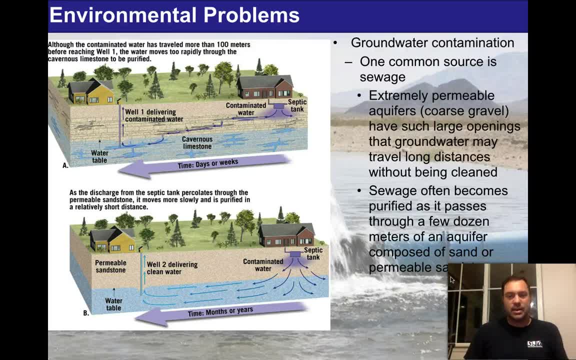 bacteria that are in the rock that will eat it. any of the waste products. that will remove a lot of the nutrients that are considered waste products. humans are, you know, it's the treasure to the bacteria in the rocks, and so septic tank, basically, the leak leaks the stuff out. it gets cleaned over time and even you. 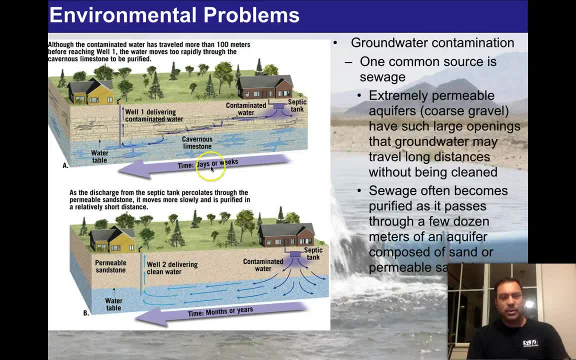 know if you have a properly engineered system- one, in this case, days or weeks. if you happen to pull it up into your water, you can actually be getting sick off of this. right, it's not getting clean. you have cavernous limestone. is transport transmitting it too quickly? so if it's taking months or years to go from point 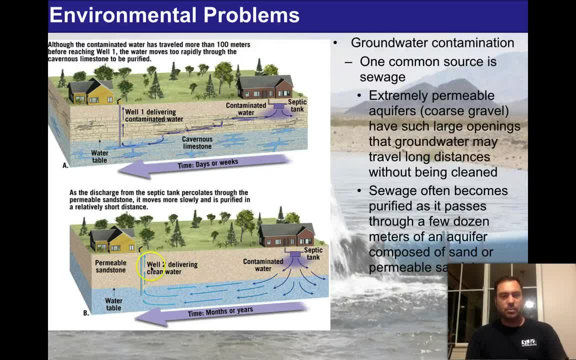 a point B, or from House ATIN House B. This water can be very, very clean. In fact, the contaminated water could be clean before it even gets to the aquifer itself. So understanding the dynamics of the aquifer and how long it moves. 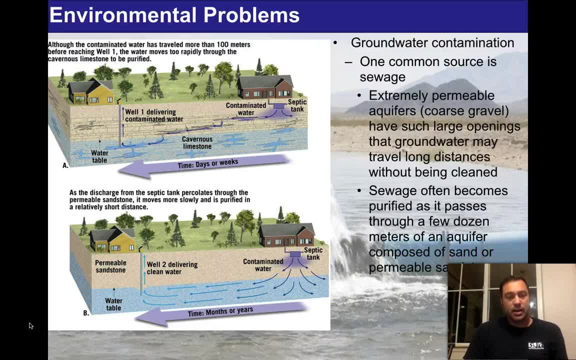 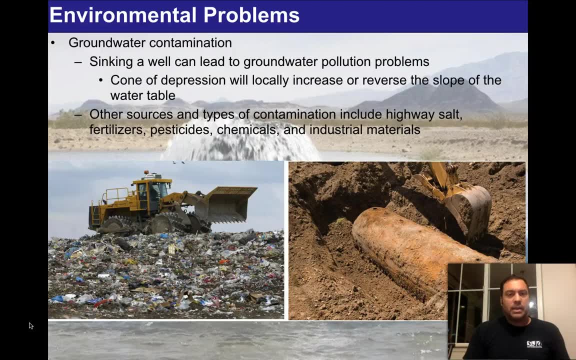 and attenuates, which is to say, to purify itself, is really, really important, And there's a whole science behind this. Another thing that we need to be aware of is groundwater contamination from different sources. right, So we have two kind of sources shown here, For example, sinking a well. 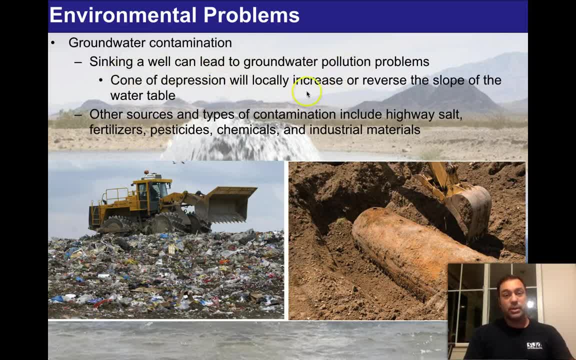 can lead to groundwater pollution problems. right, Because a cone of depression will locally increase or reverse the slope of the groundwater. So we've talked about how that can move in seawater. but the cone of depression tends to force water to go places that ordinarily would not go. 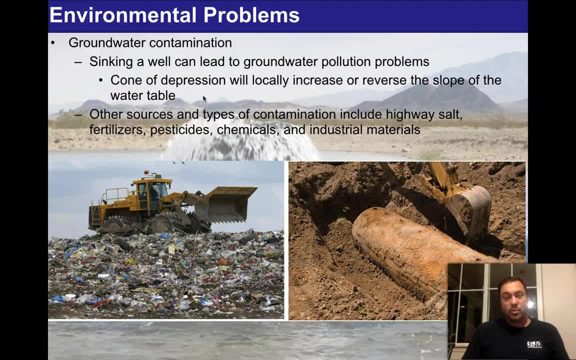 okay, So imagine a groundwater produced not too far away from, say, a gas station, and the gas station has a leaky tank. You could suddenly be drawing in water that's coming past a leaky gas tank that's buried underground. 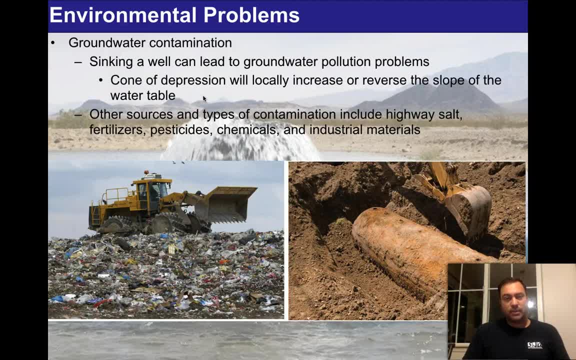 and making people sick in that municipal well. So we have to be careful of these things. Common sources of groundwater problems. This is a dump right. The water comes through. This becomes the Beto zone. The water percolates through here and anything in there, from arsenic and mercury. 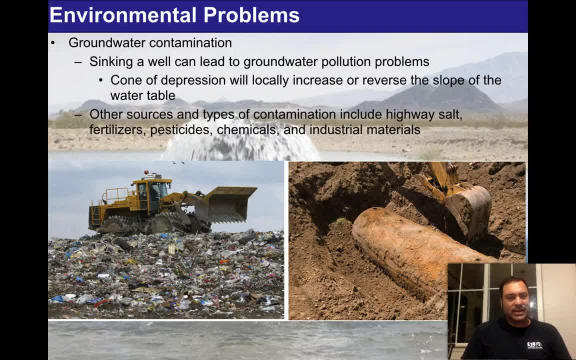 to all of the volatile organic compounds- gasoline, diesel, you name. it is going to leak down into the aquifer and do tremendous damage to the water. So we have to be careful of these things, But it's changing all the time, Right? So what can we do? What happens to this damage to the surface aquifer? at a minimum, 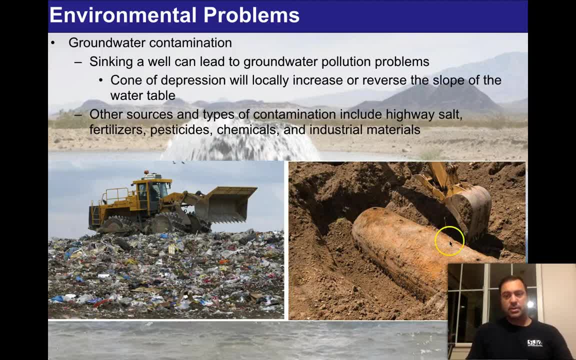 The shallow aquifer underneath the dump. This here is an underground storage tank. That is pretty typical of what we see at gas stations. So whenever you see a gas tank show up and they fill, you know, the underground tank with gasoline that you wind up buying. it usually goes into something like this and, unfortunately, 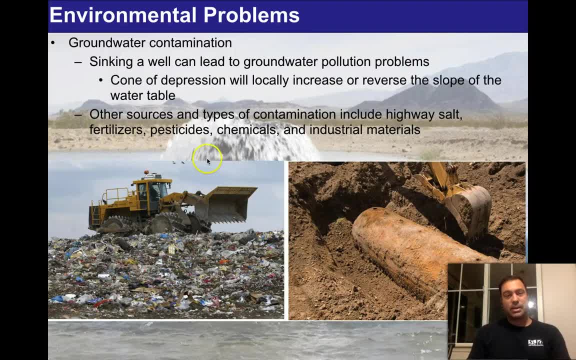 they leak a lot, okay, But there's other sources of contamination: Highway salt, right In snowy areas. that salt, That brine, winds up in the fresh water and it basically poisons the water so that people can't drink it anymore. 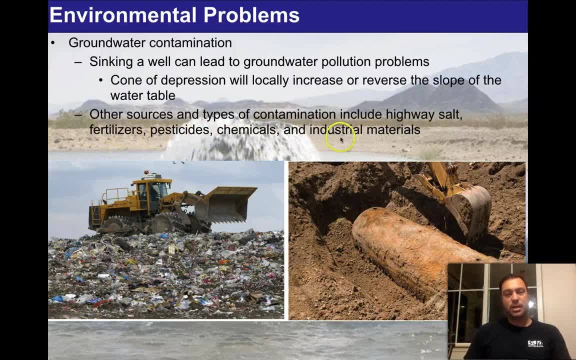 Fertilizers, pesticides, all kinds of chemicals and industrial materials. Chromium is a real common industrial material that winds up in the water, for example. It's very toxic. So you get the idea. The resources are extremely important. We're not going to go into the details of the environmental concerns, other than to say that these are kind of typical environmental concerns for groundwater. 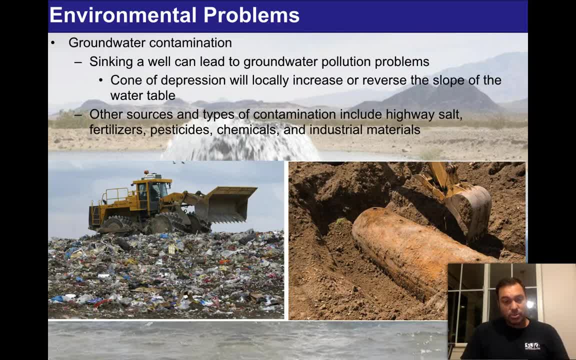 Water. 95% of our drinking water that is available to us on planet Earth, including in the third world countries, is groundwater. But a lot of it is right below our feet and we're throwing our trash on top of it, We're throwing our waste material on top of it and we're putting our fuel tanks on top of it.